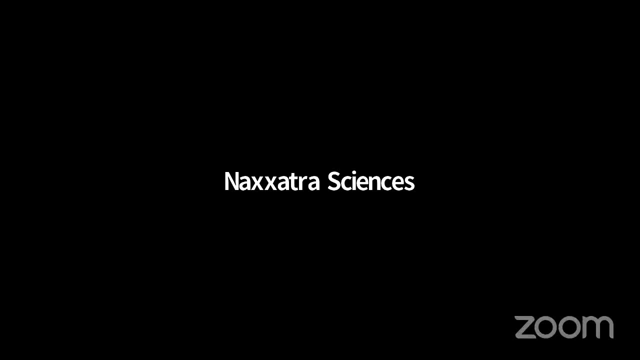 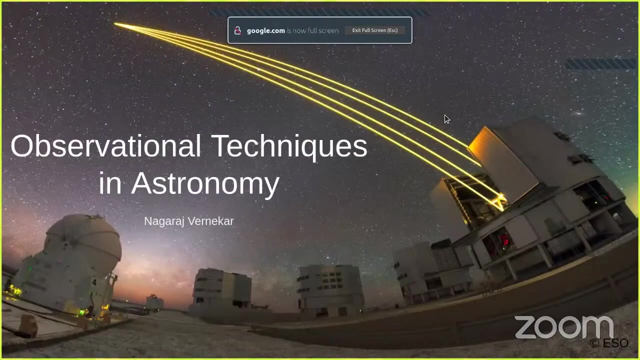 I'll just share my screen. Tell me if you can see. Hello everyone, I'm Nagraj Wernicke and I'm here to give a brief talk on the topic of observational techniques in astronomy. Before beginning, I would like to introduce: 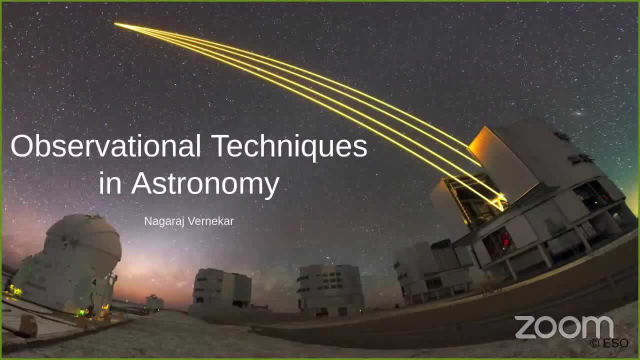 myself. I'm Nagraj Wernicke. I'm the Director of the Institute of Astronomy at the Institute of Astronomy at the University of London. I'm a master degree student from KU Leuven, Belgium. I have specialized in the topic of astronomy and astrophysics in my master's with an interest. 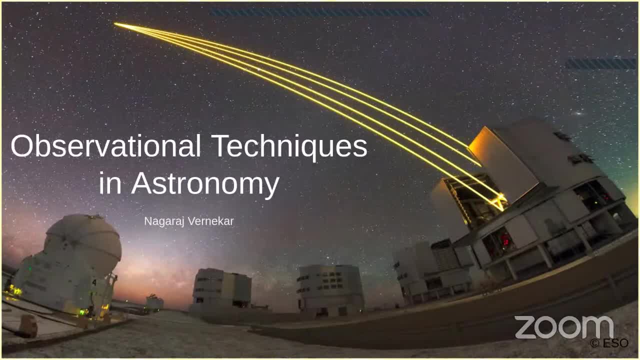 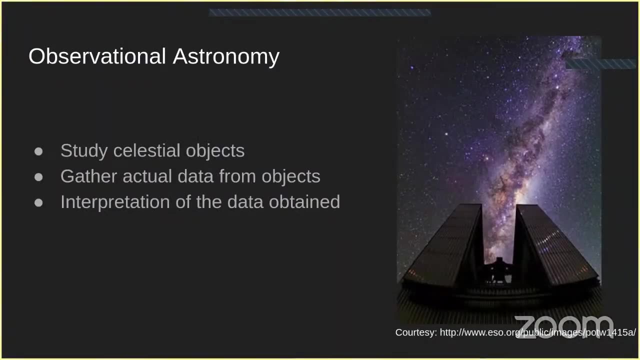 in stellar evolution and stellar structures. Currently, I am a research assistant at the Indian Institute of Astrophysics, working on massive star formation. Let's start now. So what is observational astronomy? Astronomy is a wide field. It is further divided into three different subtopics. which is observational astronomy? 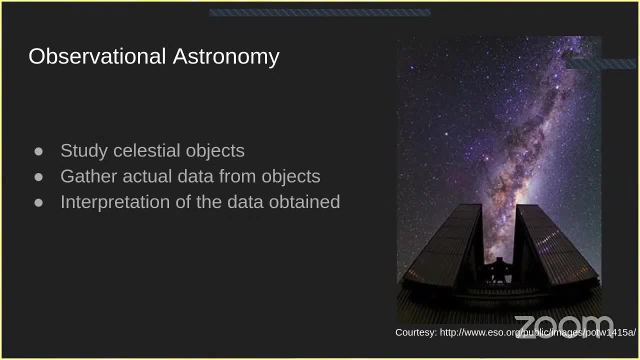 theoretical astronomy and computational astronomy. In observational astronomy, the astronomers try to study celestial objects like stars, galaxies, supernovae, by collecting the data from these objects using different instruments like telescopes, interferometers etc. And then look at the observed data and interpret what might be going on in that star which. 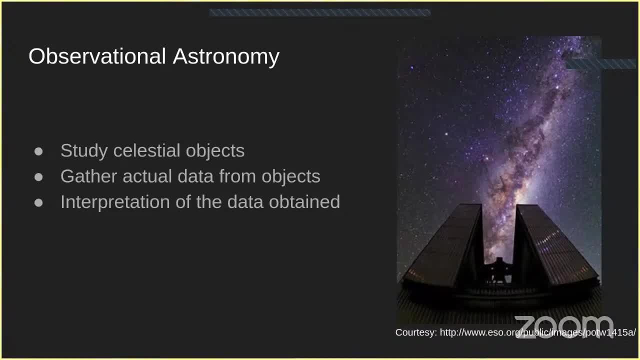 is why we are getting the particular data that is observed. This is the gist of the entire observational astronomy. When someone puts it like this, you might see it. It might seem that it is pretty straightforward, that you just take the data and you look at. 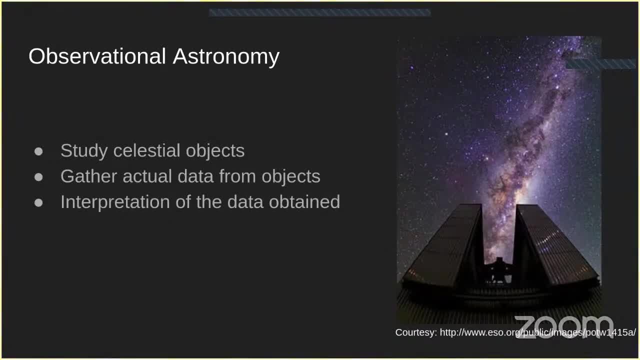 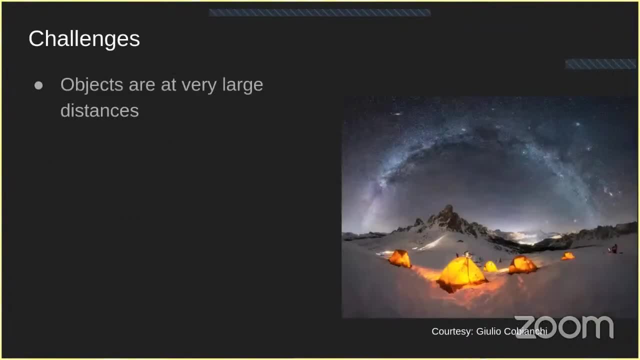 it and see what's happening. But like everything else, there is a lot of challenges that one has to face when you're trying to do something. The first challenge is: the objects that you're trying to study are really really far, far away. 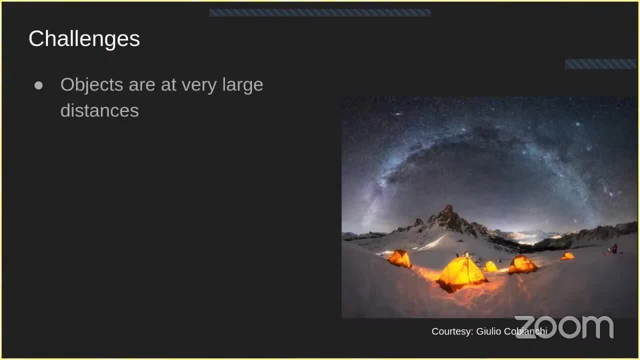 Like you know, that the universe itself is so large and it has billions and billions of galaxies, And each galaxy has billions of stars, And each of the distance between each of these stars is so large that it's beyond imagination. Here in the photo you can see the galactic disk of the Milky Way. 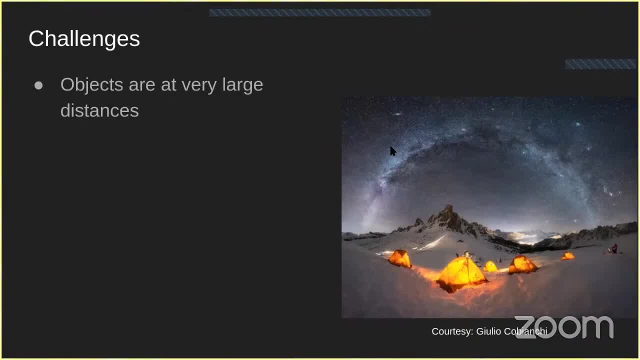 And just to try to realize how far these distances are, you can see that the center of the Milky Way, which is the supermassive black hole in the center, Sagittarius, is just a little center. Sagittarius A is around 26,000 light years, So light itself takes 26,000 years. 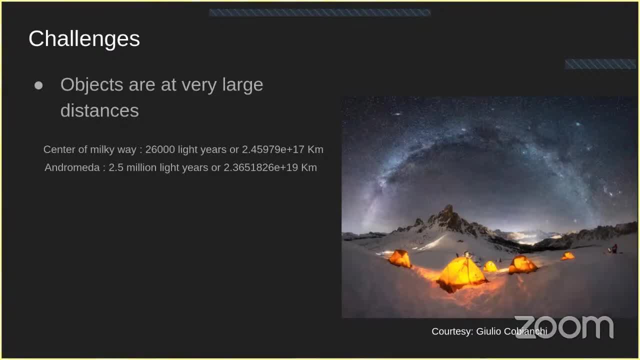 If you want to put that in the units that we use in everyday life, it's 2.4 into 10 to the power of 17 kilometers. We never come across such a large number in day-to-day life. but yeah, this is the distances that you're working with And in this image you can see a small speck of. 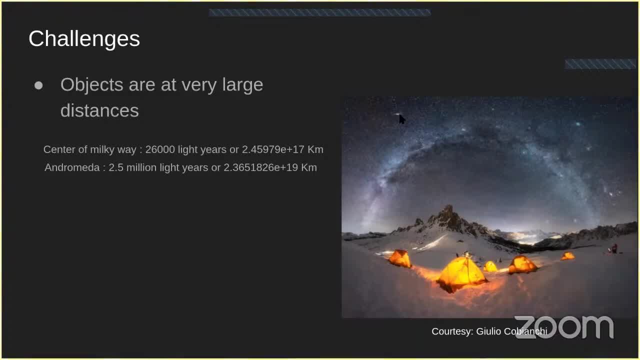 a blurred kind of an image here, And this is actually the Andromeda Galaxy, which is the closest galaxy to Milky Way. But even though it's the closest, it's still 2.5 million light years away. In kilometers it's around 2.3 into 10, to the power of 19 kilometers. That's like 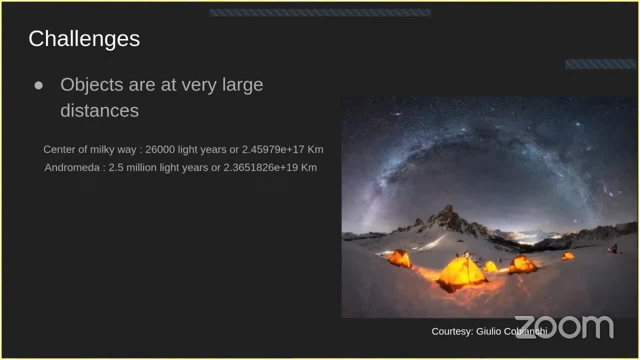 a quintillion kilometers, which is immensely large. But there is one good news: that Andromeda is a coming closer to Milky Way, So in a few million years you might even be able to visit it if you are alive. The second difficulty comes because of the distance itself. Let's take an example of a. 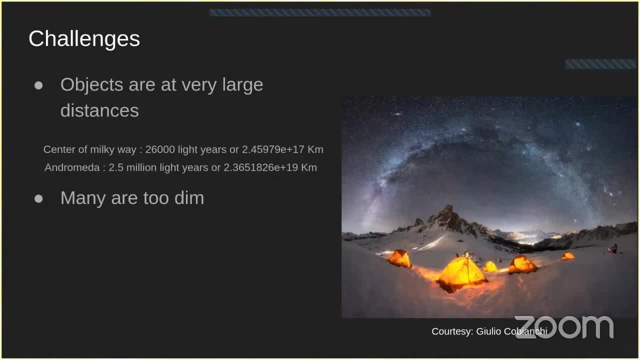 star. A star radiates energy and it radiates in all directions equally. But because so when the distance is from the star? That's exactly what I wanted to say. Sorry, Yeah, Okay, So as the distance from the star increases the total flux that you 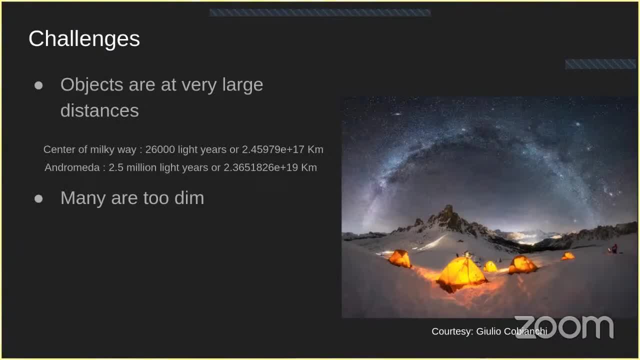 observe from Earth is a very small fraction of the lumina, of the flux that the star actually emitted. All the other percentage of the flux just goes away in every single direction. So, due to these immense distances, the flux that you observe is very, very small, And this is So when. 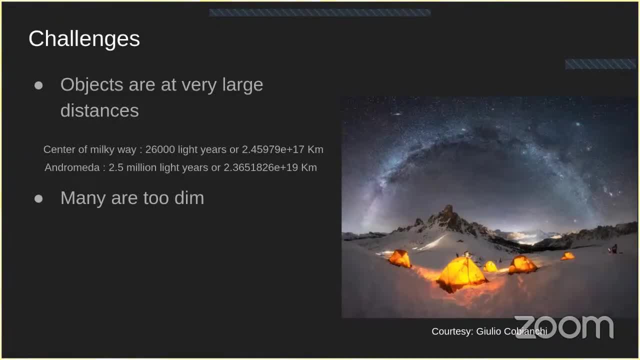 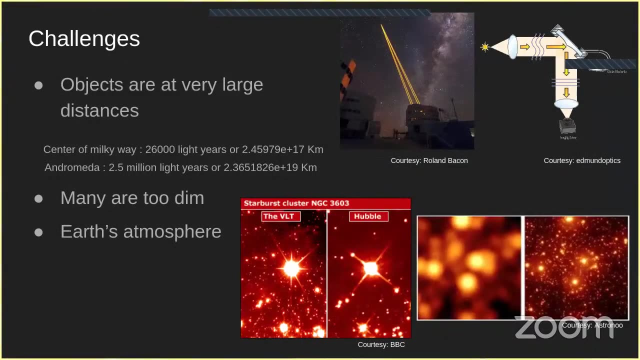 you're observing something like other galaxies. the light is, The number of photons that you observe is so short that you need to take very long exposures, And that kind of adds into the difficulty of trying to analyze certain objects. The third difficulty is very close to us. 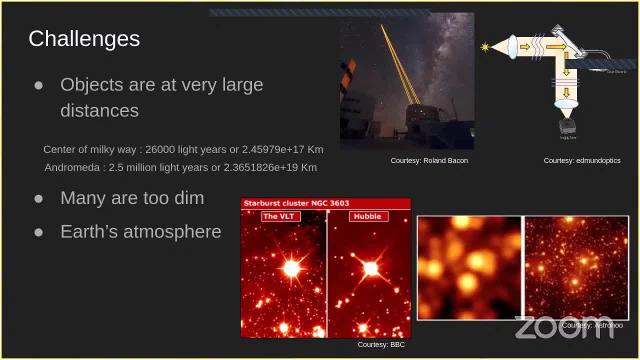 It's the Earth's atmosphere. So Earth's atmosphere, even though it's very good for humans- it gives us protection, It gives us Oxygen and everything- It is a bit. It makes an astronomer's life very difficult because Earth's atmosphere it's not static, So it's not same all the time Earth's atmosphere is. 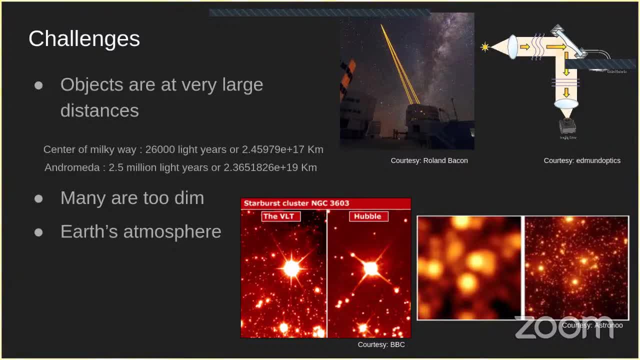 very dynamic that it changes. There is like wind flowing. So the density of the layers of the atmosphere changes constantly and very fast. So when you try to observe- so you have a ground-based telescope and you try to observe the light from 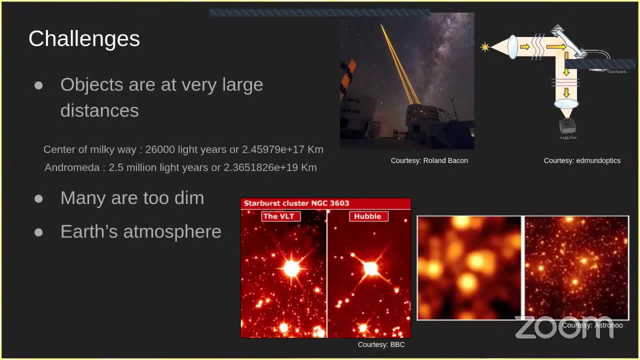 The light. actually, it shifts due to the difference in the atmosphere. You could have seen it from Yonekera itself, that stars twinkle. You can see stars twinkling in the sky. That's not because the star is doing something, but it's because the Earth's atmosphere is very turbulent. 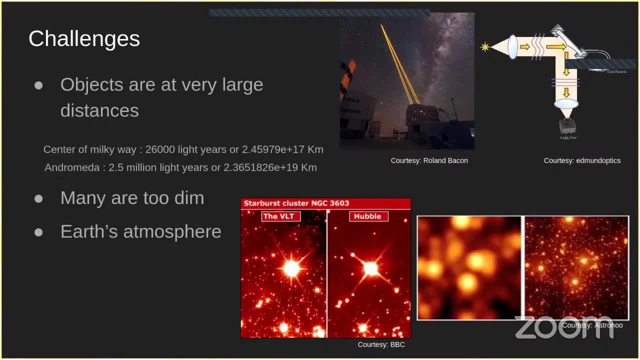 And when you try to observe, when you observe something in the turbulence of the Earth's atmosphere, then this is the image that you get It's. You can just see the blurriness in the image that you get and you can just see blobs of light everywhere. 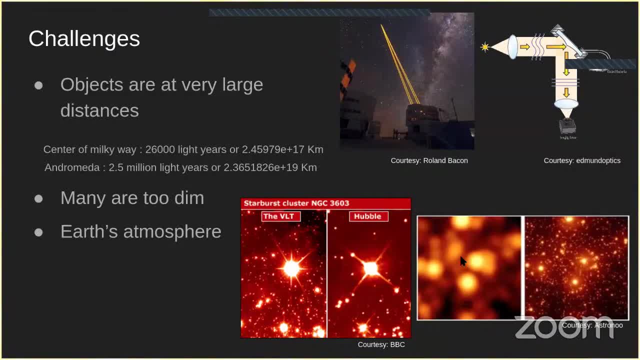 This can still be used to study certain, certain phenomena, but there's a limit to what you can do with this image And with the current day level of research. this is not enough. This type of resolution is not enough. This type of sharpness in the image, 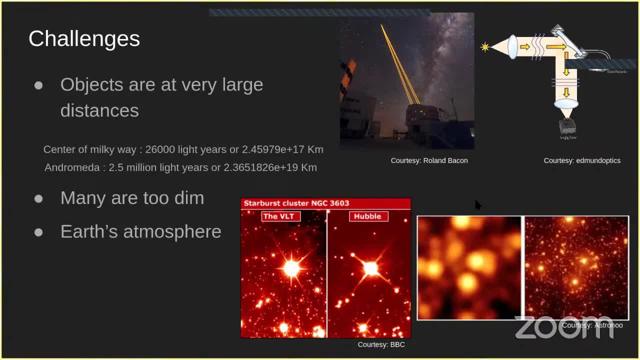 So they have come up with an ingenious solution which is called adaptive optics, where they artificially first create an artificial star using lasers. as you can see, This is the very large telescope from European Southern Observatory, So you can see the laser shooting up. 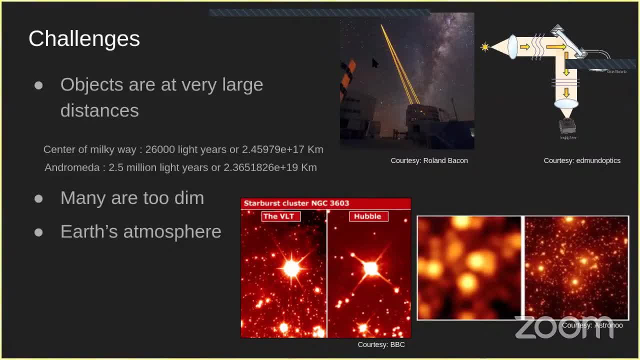 and it creates a artificial star in the field of view And then they look at that star. It gives an idea of what the atmosphere is doing And then they correct that, that disturbance, using a flexible mirror where you can change the curvature of the mirror. 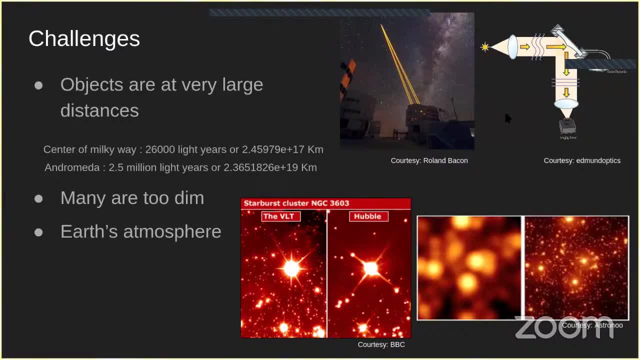 based on your inputs, And this is done tremendously fast because the atmosphere changes so quickly. This whole technology is called adaptive optics, And here you can see a real life example of how adaptive optics increases the resolution of a telescope. You can see that the blobs just become really good. 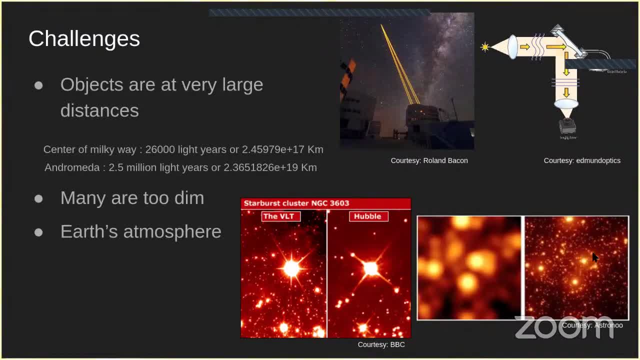 just become really good, just become really good, good stars, like they're really finite, Coming to the level of improvement that adaptive optics brings. you can see that here. it's the BLT, which is the same telescope. You can see the image above. 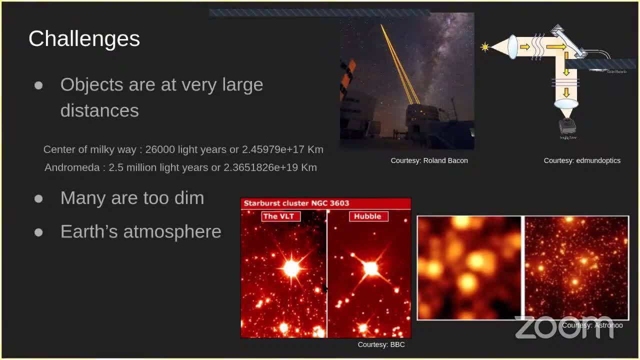 which is the very large telescope. The resolution of BLT is comparable to the resolution of Hubble, which is a billion dollar space telescope. So using this technology, you can build much, much, much, much, much larger ground-based telescopes. 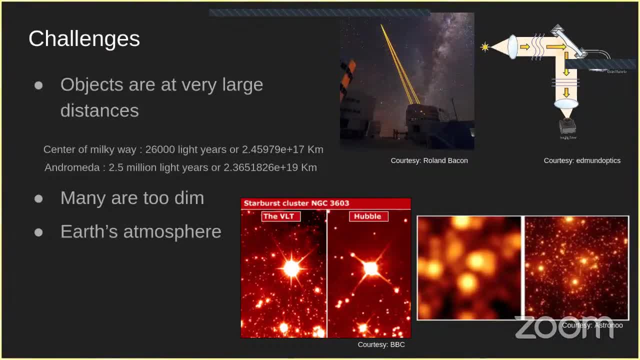 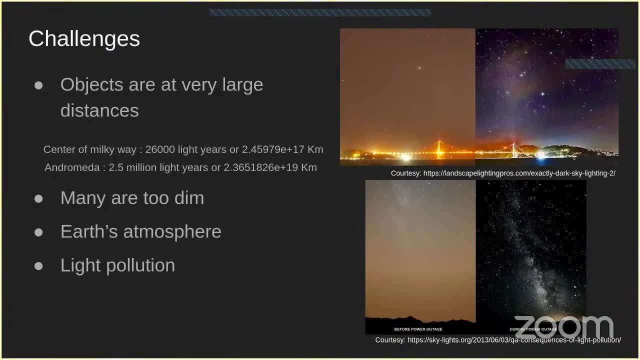 which have a resolution better than the space telescopes, because launching space telescopes is a tremendous task and also takes in a lot of money. The fourth challenge is the light pollution. As you know that if you live in a city anywhere in India, 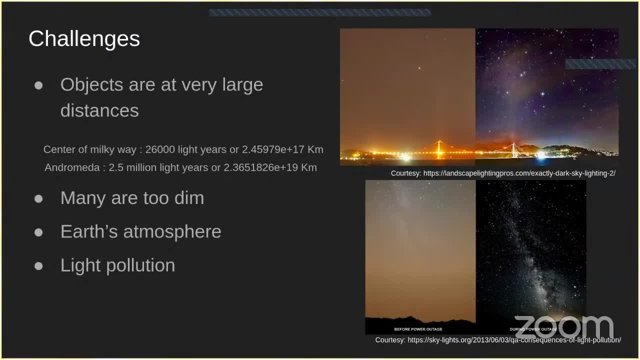 you barely see a few couple of stars in the sky, but in reality, this is what you need to see. So if there was no light pollution, this is what you see. This is what you would have seen every day, every night. 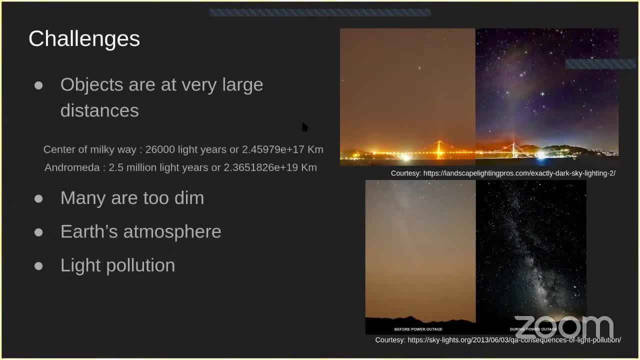 But because there is so much light usage in the cities, it illuminates the sky, which then reduces the visibility of telescopes around the world. So there is not really any way to correct light pollution. You can use filters, but again that will increase the exposure times of your observations. 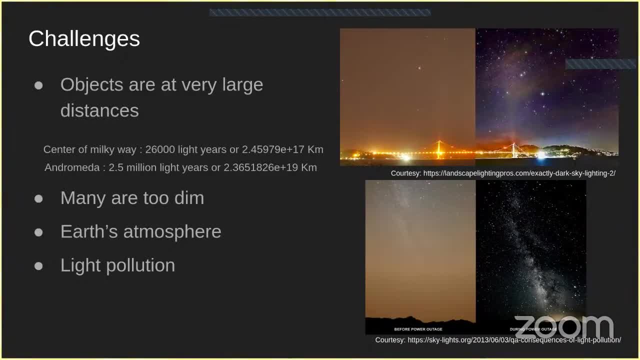 which is not a good solution. So the only solution that currently is used is to build all the telescopes away from cities and everything like that. Currently, there are a handful of hotspots around the world where telescopes are built because of their pristine conditions. 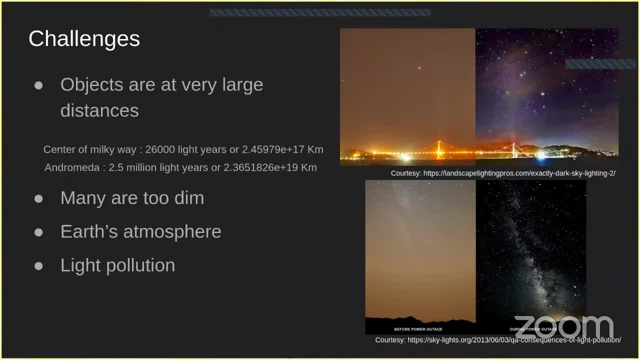 One of them in India, it's Ladakh. So there are a few telescopes in Ladakh where people observe from. There is one in Mount Ikea, that is USA, And the The biggest of all is the Atacama Desert in Chile. 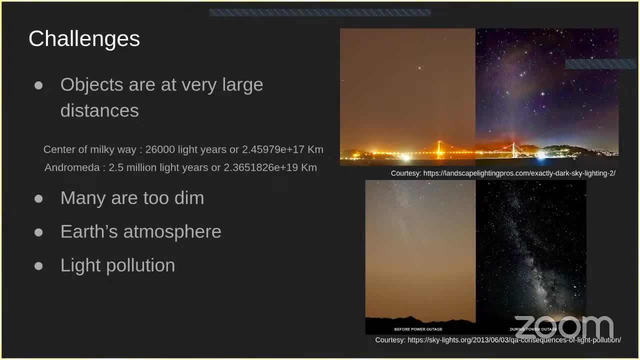 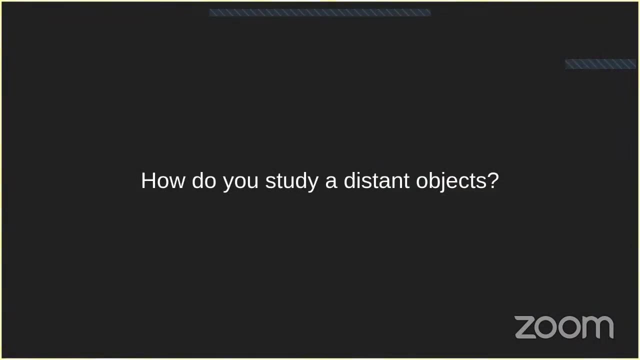 where there are, like one of the world's biggest telescopes situated, like the 40 meter extremely large telescope, the giant Magellanic Telescope and also the ALMA radio telescope. So I have addressed the third and the fourth issue of how astronomers try to solve it. 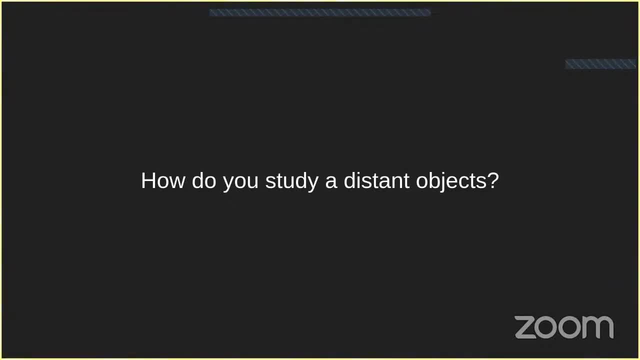 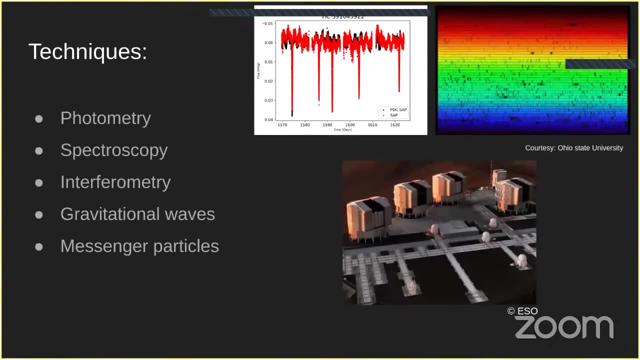 but there's still the first two issue that the distances and the brightnesses. So how do we actually solve it? How do we actually study these such distant objects? There are a few techniques that we use. Each of these techniques gives a different. 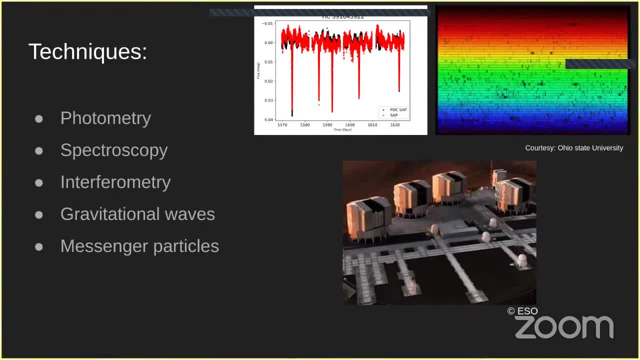 Each of these techniques probes a different phenomenon. So there are like five different techniques here. So first one is photometry. Photometry is the simplest one. I feel that it's the simplest one, where you just monitor the brightness of the star that you see. 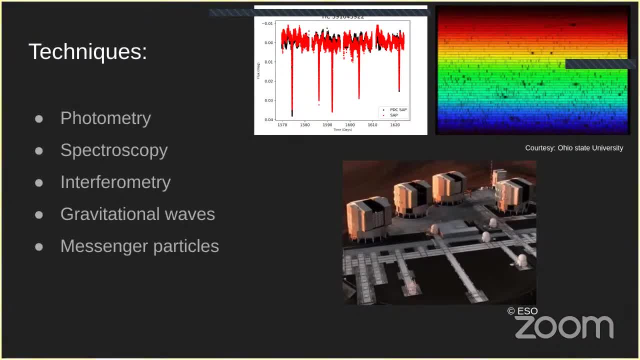 That's what you're looking at, So you just constantly take observations and see how the brightness of the star changes. Here is an example of an eclipsing system. So there are two stars which go around and they eclipse just like the sun and moon does. 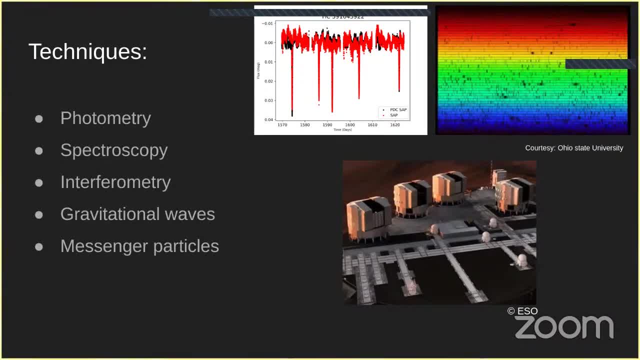 sun, earth and moon does with each other. So when the eclipses occur, you can see that there's a dip in the light curve, And these are periodic. even though they don't seem periodic, they are, this is because it's an eccentric orbit. 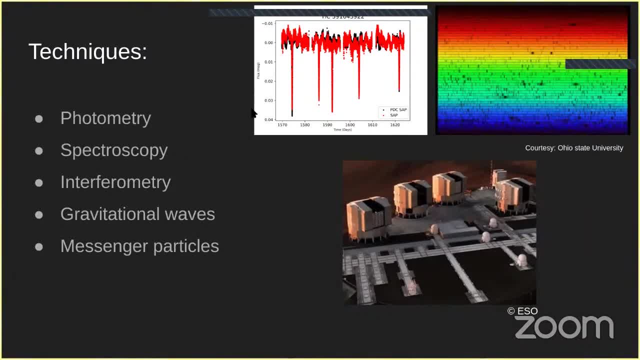 but yeah, this happens in a periodic fashion And you can, by just looking at it, you know that there are more. there is more than one star in that system. So this is quite useful And you can also study it. So you can see, here there is a lot of variation. 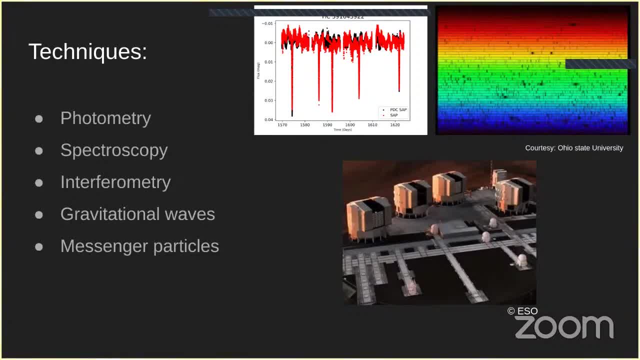 So there's upturn, upturn, upturn. This is the pulsations in the star. So the star is a way like the radius increases and decreases in time with respect to time, And that causes certain changes. Why this occurs? 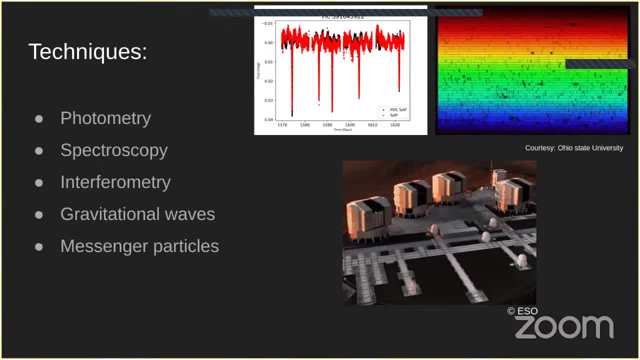 It's some internal mechanism which is a complicated subject which we are not going into. The second technique is spectroscopy. So spectroscopy is a technique where you take the light from the star and then you split it into all the constituent colors. 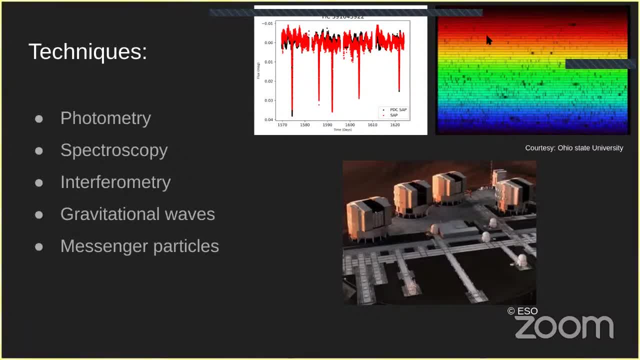 So you split the light that you get and into a spectrum. So this is what a usual spectrum of a star looks like. You can see that there is like the, that you see the rainbow thing. So there's red, there's yellow, there's green, there's blue. 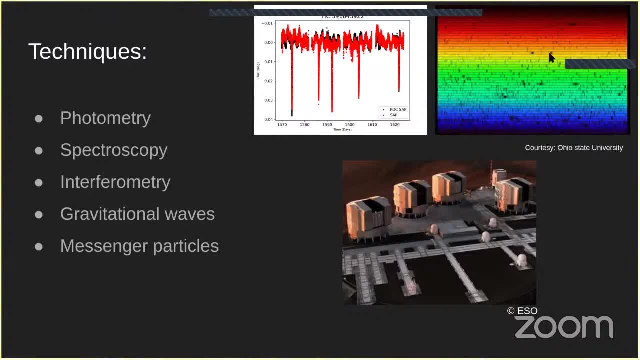 But along with those colors, you can also see some black lines in between. So there are many black lines, like a lot of them. So what are these These are actually? so it's not a continuous spectrum. This is because star is made up of many different elements. Like, the most abundant are hydrogen, helium and oxygen. So these are actually, so it's not a continuous spectrum. This is because star is made up of many different elements, Like the most abundant are hydrogen, helium and oxygen. So these are actually, so it's not a continuous spectrum. This is because star is made up of many different elements. 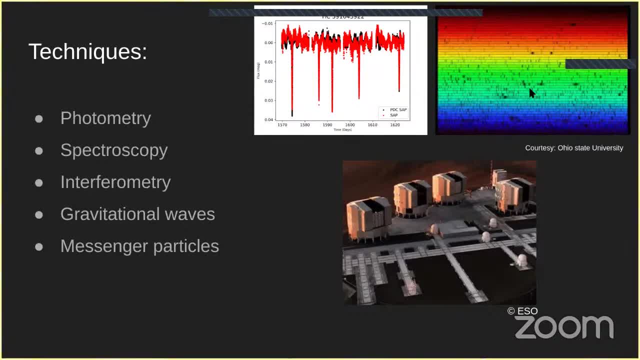 So these are actually. so it's not a continuous spectrum. This is because star is made up of many different elements, So when the light travels in the star, these elements absorb certain frequencies of light. So when the light travels in the star, 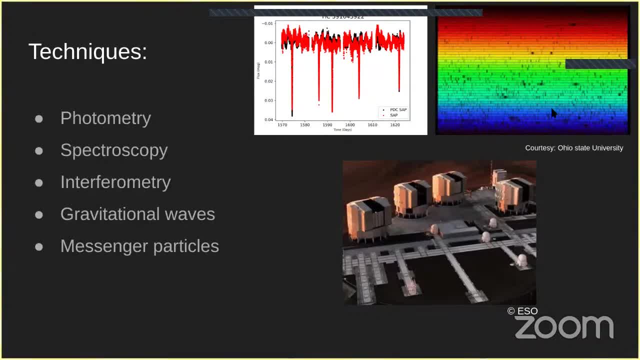 these elements absorb certain frequencies of light And when they absorb the light. these elements absorb certain frequencies of light And when they absorb the light, it no more reaches you, right. And when they absorb the light, it no more reaches you right. 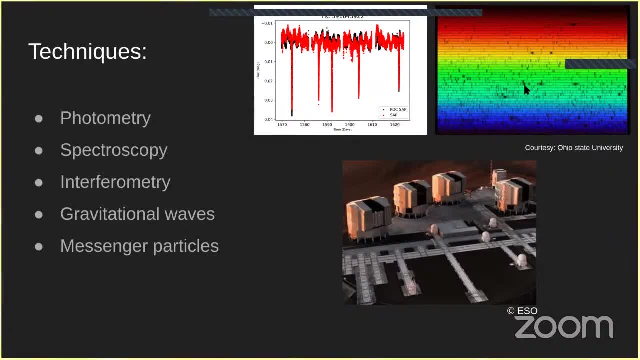 So at those particular frequencies you don't get any light, and that is represented by the black color here. it no more reaches you right. So at those particular frequencies you don't get any light, and that is represented by the black color here. 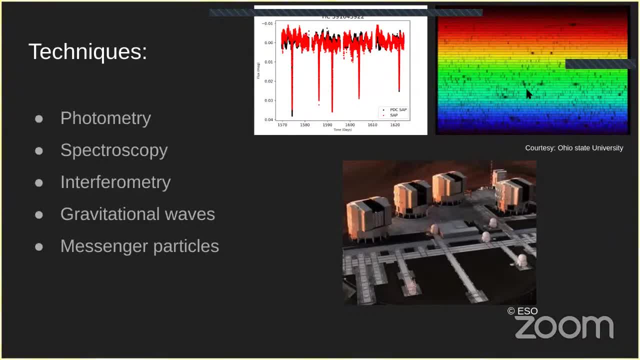 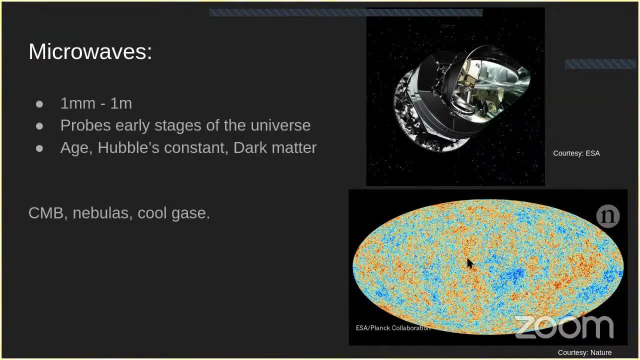 And you can study these spectral lines to actually know what kind of composition the star has. And you can study these spectral lines to actually know what kind of composition the star has like. not, it's not a smooth thing, so there is many differences and it is. it is interesting to know why. 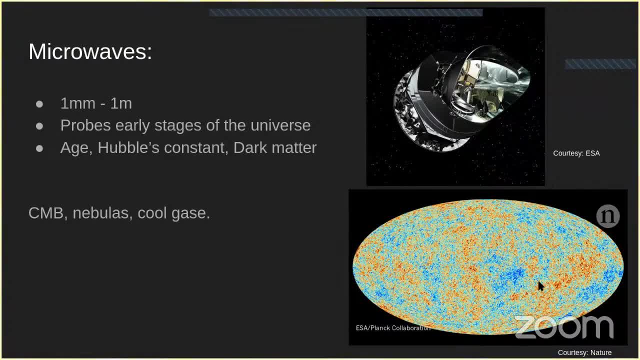 there is difference and also cmb was used to measure the age of the universe, also the hubble's constant and probe, the dark matter, which is again a very mysterious topic for now. so microwaves have been useful in finding, in studying more about the early universe, early stages of the universe. 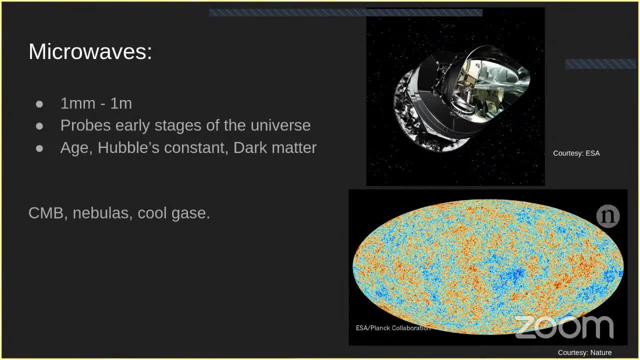 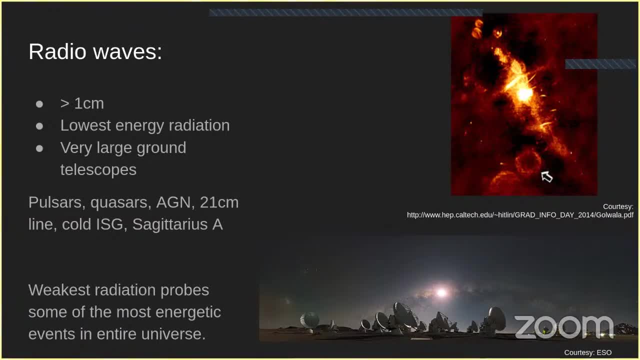 and also estimating the age of of the universe. the last ones and the last and the least energetic radiations are the radiowaves. these are the waves which have wavelength longer than one centimeter and, again because they have such long wavelengths, they are very low energy radiations. 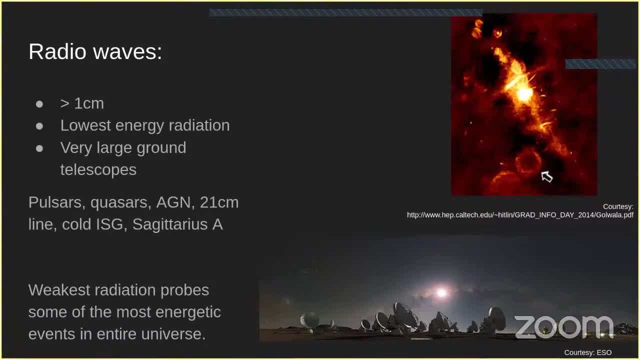 uh, earth is. earth is very transparent to radio waves, so majority of the observations are done by ground based telescopes. Here you can see that uh. here you can see a photo of ALMA. ALMA is a. again, it uses interferometry techniques, so there are like many different uh many uh antennas that absorb that uh. 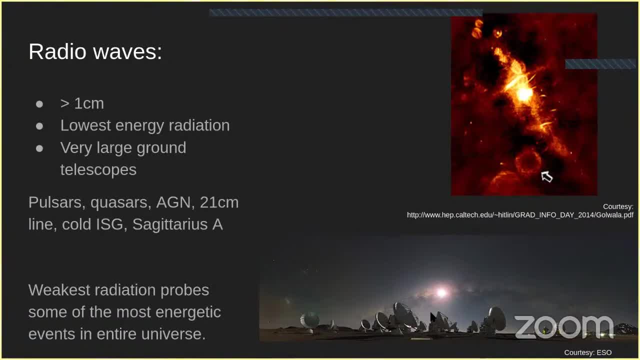 that absorb the radiations. and then there the data is come together: Uh, this, this radiation is especially important because these radiations are emitted from sources like pulsars, like the pulsars are nothing but neutron stars, with, with the jet uh coming out from it Like AGNs again. 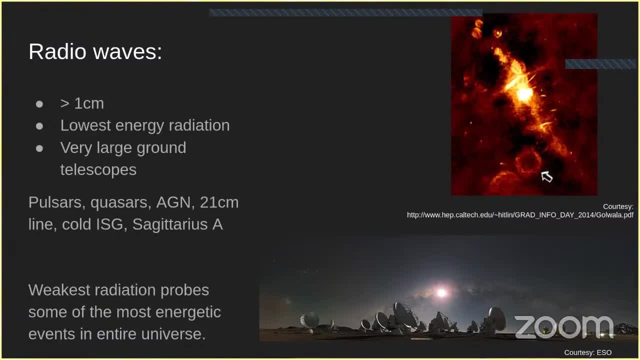 active galactic nuclei, the black hole in the in the center of galaxies, The Sagittarius A, which is the supermassive black hole in the center of milky way. So, even though these, even though radio waves, is one of the weakest uh energy uh, weakest uh uh electromagnetic radiation in terms of energy. 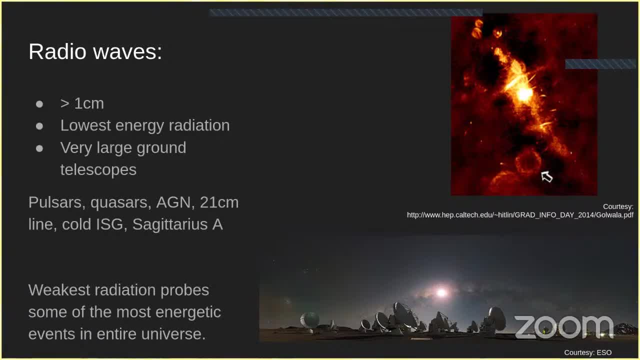 it's, it still helps in probing one of the most violent events in the universe. So this is extremely fascinating, that something so weak can actually probe so energetic events. At least I was surprised when I knew this for the first time. Uh, here is an, uh a radio image of uh the Sagittarius. 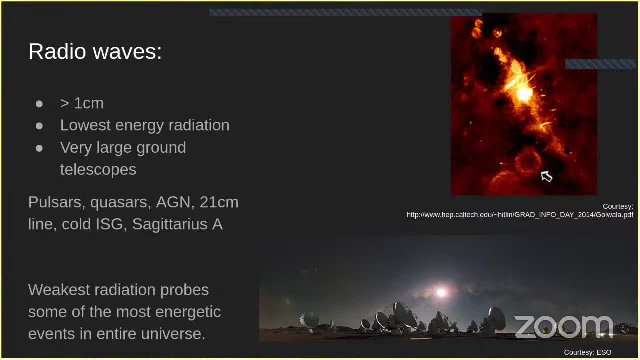 A star, Sagittarius, A star so center of milky way, and uh, in the arrow it shows, uh, it's showing you, uh, so you can see a cloud kind of a thing. that is the supernova remnant of a star that went boom, uh in in, uh in the recent past. Uh, yeah, so at the last one is visible light. uh, visible light as you. 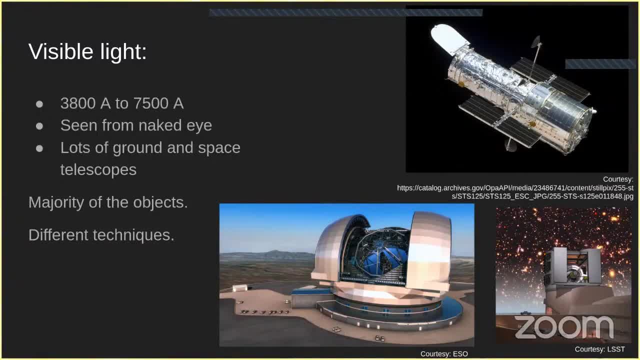 uh, as you know, is is the region between the blue light and the red and the red light, or the violet light, between the red light, and it has a wavelength of 3800 and songs to 7500 and songs. This is the only light that has us as humans can see. uh, we cannot see the other radiations. um, uh and uh yeah. 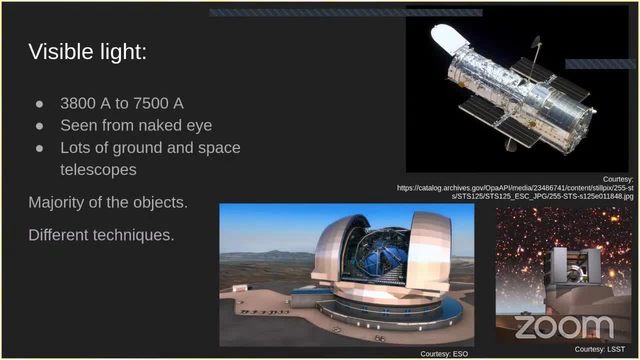 so this is a why. so this is where a lot of astronomy happens. because, again, you can. you can build telescopes on land and you can go to space. Some of the examples are: some of these examples of space telescopes is the Hubble, which is the iconic uh image here. um, it has done a. 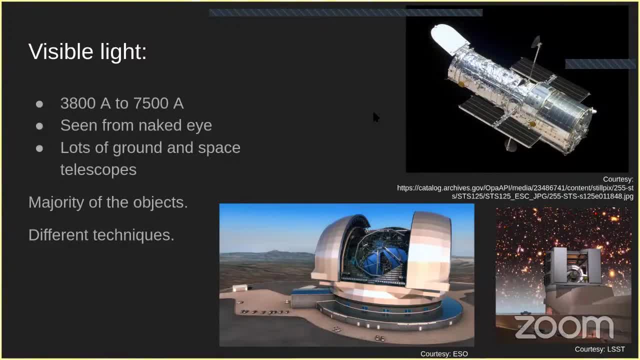 remarkable uh contribution to the field of astronomy. uh, especially, uh, uh. you might have known the deep field image which kind of gave us an idea of how, how large the universe is. Some of these are some examples. these are some examples of ground-based uh telescopes, the, the, 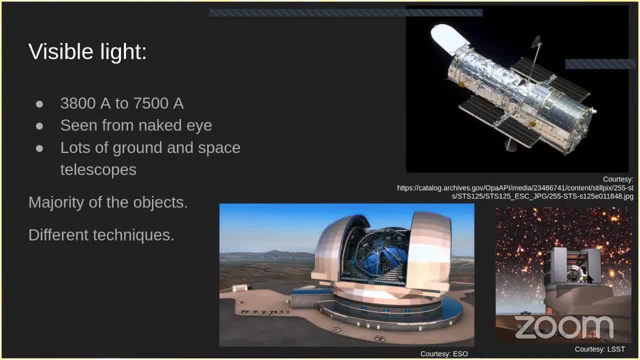 one on the extreme right is the LSST, which is a survey telescope currently being built, so this will survey the entire sky, uh in in like 10 days, so it'll keep doing it for a long period of time. so it'll help in finding a. 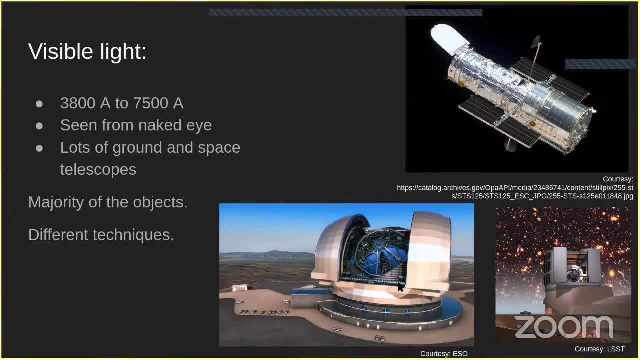 lot of asteroids and many different kind of changes in the universe. uh, as a matter of fact, this has the largest camera ever built for any purpose. uh, on the on the left uh is the extremely large telescope from european space southern observatory. this is being built in? uh, chile, Atacama desert and. 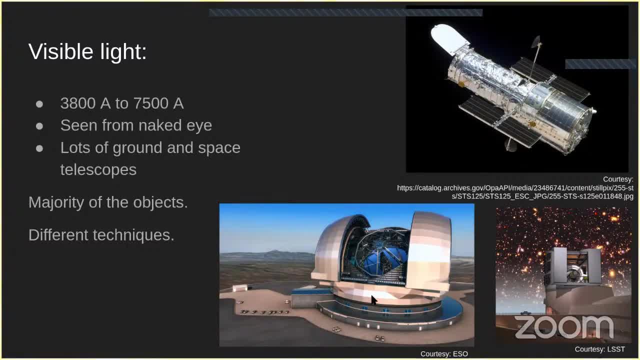 it has a primary and a secondary telescope. This is a very large telescope and it has a primary mirror of 40 meters, which will be the largest mirror ever built, and so this telescope will will will have a really good resolution to do a lot of science. 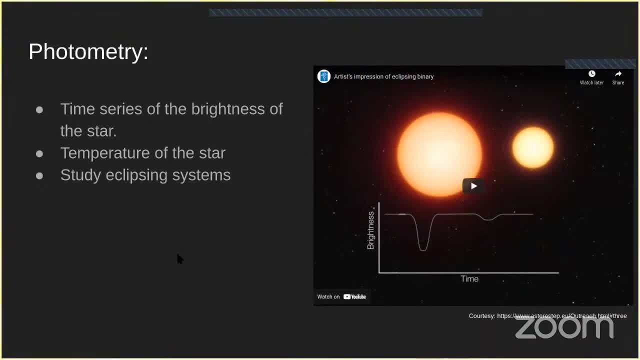 So, yeah, let's just go in depth of the different techniques that I mentioned. so first, let's start with photometry. as uh explained, photometry is just a time series and you measure the brightness of the system, And I also showed you an example of of of the eclipsing system that I showed uh. photometry can. 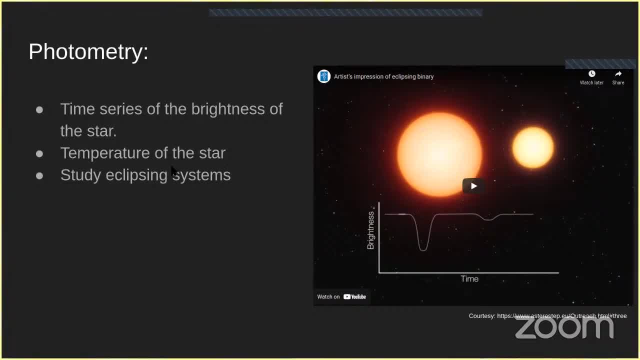 be used to uh estimate the temperature of the star uh. this cannot be directly done through the time series. instead you use something called as SED, which is a spectral energy distribution. so you it kind of gives you an idea where the highest emission uh is in the in the wavelength region. 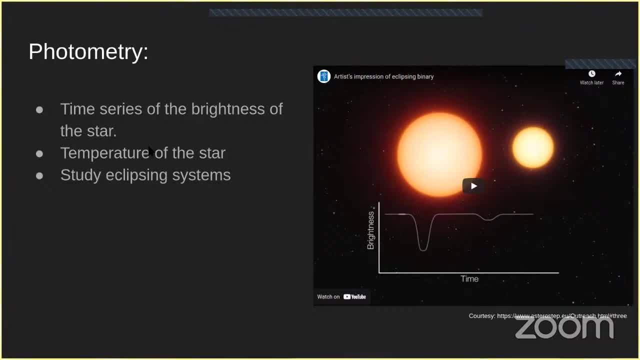 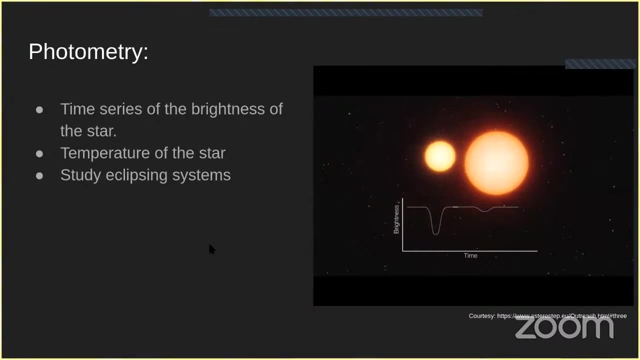 and through that you can kind of estimate what star you are dealing with. uh, it helps in studying eclipsing systems. uh, as the example showed. I'll show you why. uh, why, here is a video from ESO so you can see that the two stars are eclipsing each other, and then 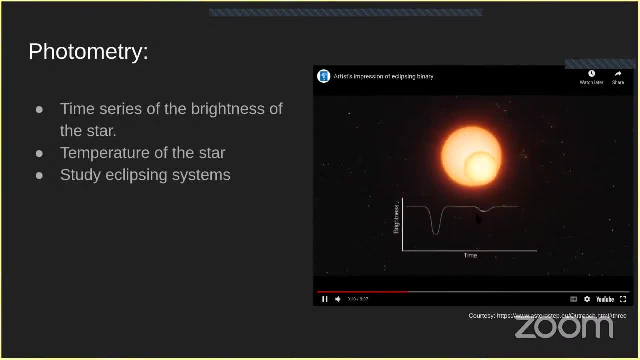 here is the light curve that you will get. so this is the theoretical, but, yeah, this is what you would. you would initially find. so when it eclipses, the, there is a dip in light curve, and when the other star comes in front, the- the eclipse depth changes. so by doing this, 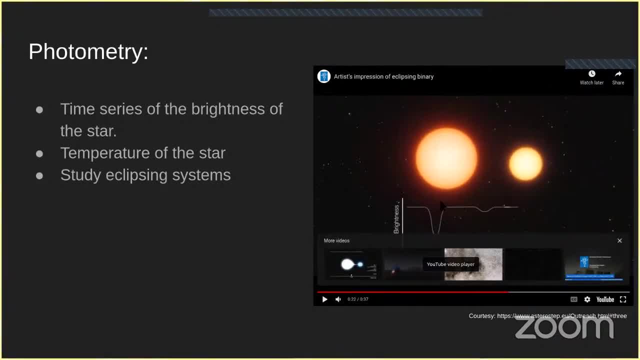 By probing. so by studying this eclipse depths and the difference between the two eclipses, you can find many parameters like how massive the star, what is the radius of the two stars, what are the masses of the two stars, what are the temperatures of the stars, and many. 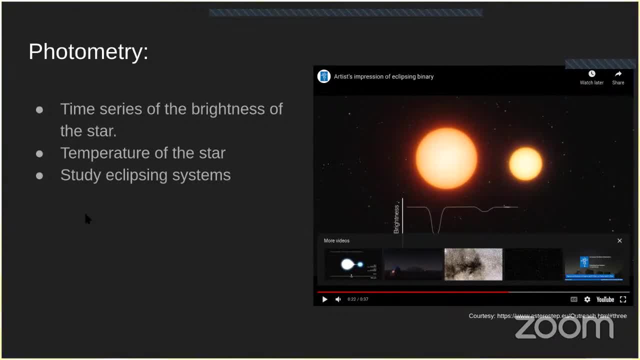 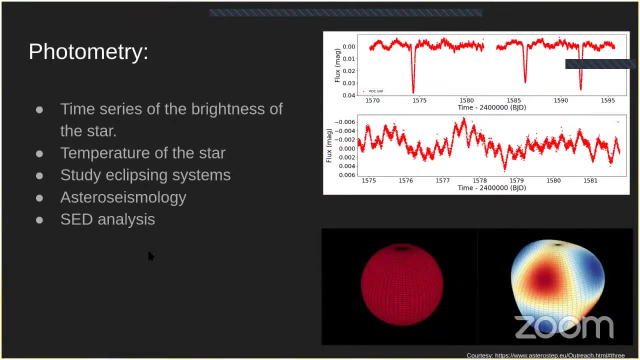 more things like that, which is extremely useful in categorizing these systems. The other uses of astronomy, of photometry, would be something called astro seismology. Astro seismology is a field where we study the star quakes, so like earthquakes even. 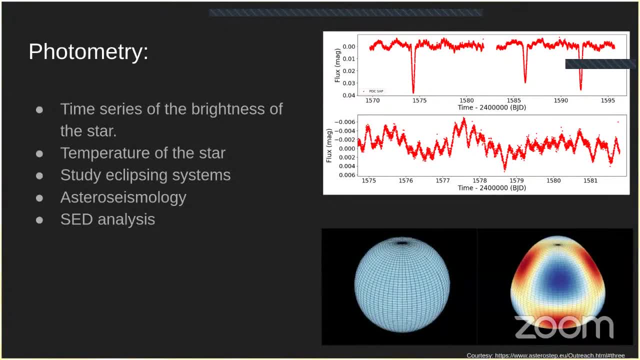 stars have quakes in them where they kind of move, the surface moves. Here is an example of like two examples. So these are different kinds of motions. You have a lot of different kinds of motions in a star. The first one is the simplest one, where just the star increases, the radius increases and 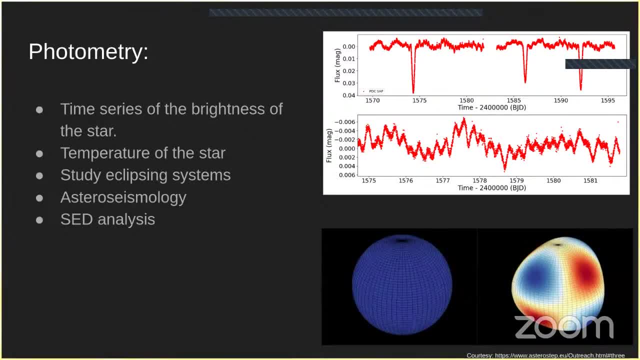 then decreases and increases and decreases. This happens periodically. And the second one is quite a complicated motion. The blue regions indicate the surface which is towards you, So it's like it's coming away, like it's coming towards you, and the red region indicate the. 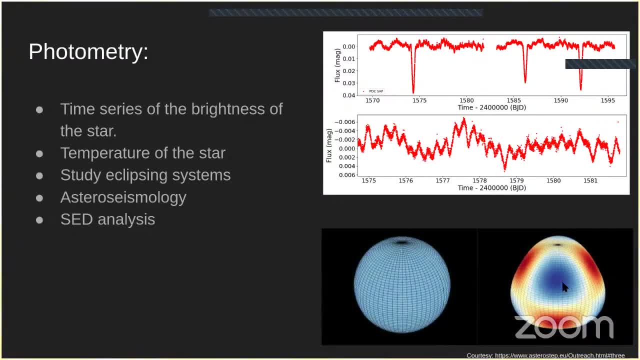 ones that are going inside. So some regions are bulging outside Whereas some regions are bulging inside, And this happens again periodically. The reason for these things to occur is, again, certain phenomenons happening inside the star, certain instabilities. You can, if you want, you can just go through astro seismology and you'll find a lot of. 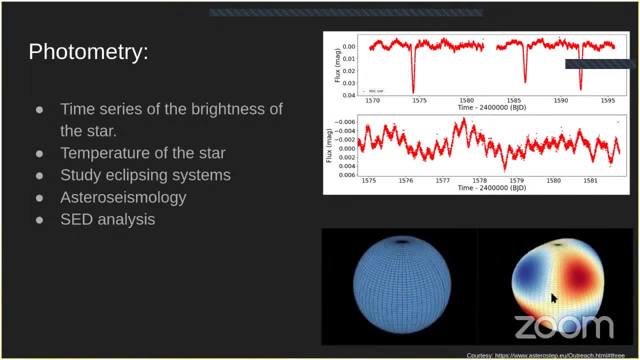 material, if you're interested. And so this kind of variation in the star has an effect on the brightness that you see in the light curve. So this is an example light curve of the same eclipsing system, But like if you remove the eclipses in between and you just concentrate on the on the out. 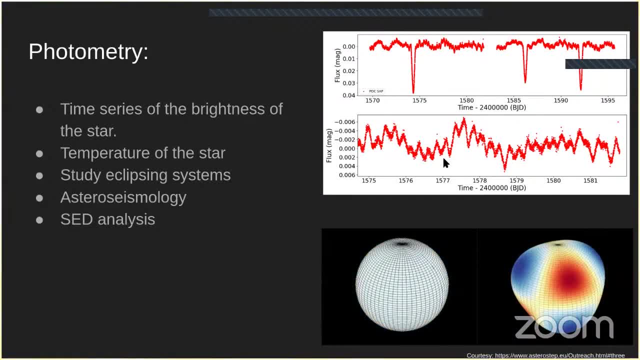 of eclipse region. you can see that there is a lot of variation in the in the light curve. It keeps going up and down, up and down, up and down, And like it might seem that they they are just random, but these are actually a lot. 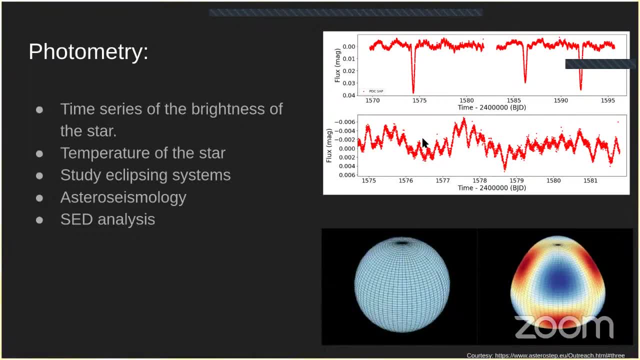 of periodic variations having a constructive interference with each other and then forming these systems, Forming these variations. You can study these variations and then kind of analyze what, what the star is doing and also probe the interior of the star, including the core of the star. 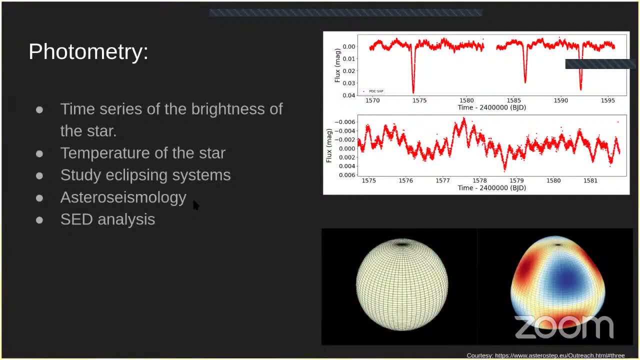 That is why astro seismology is such a such a useful tool. because, no, because you cannot see the core of the star directly, So you cannot see inside the star directly. So astro seismology gives you an indirect way of studying the interior of the stars. 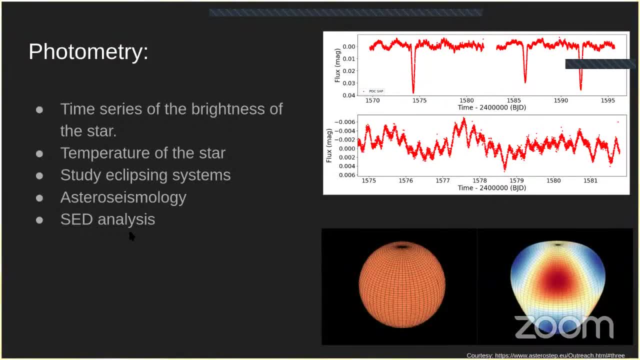 Again, SED has explained, kind of gives you the temperature of the stars, the temperature of the star, and you kind of, you kind of know what kind of system you are dealing with. Coming to spectroscopy, spectroscopy, again, you split the light into constituent colors. 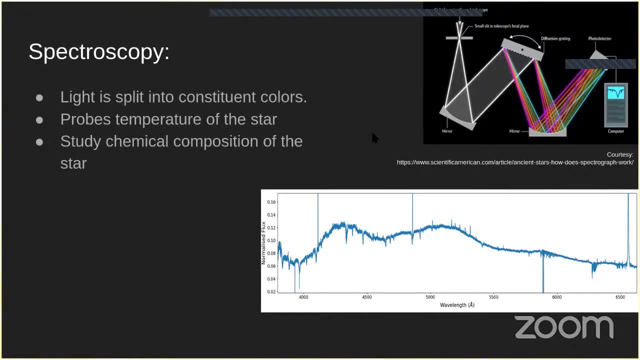 and then you study the spectral lines to see: So how do you split? So this is a kind of representation of a spectrograph, of a very simple spectrograph. So there's a slit through which the light comes out, Okay, So the light comes in. so there's a telescope, and then the light comes in through the slit. 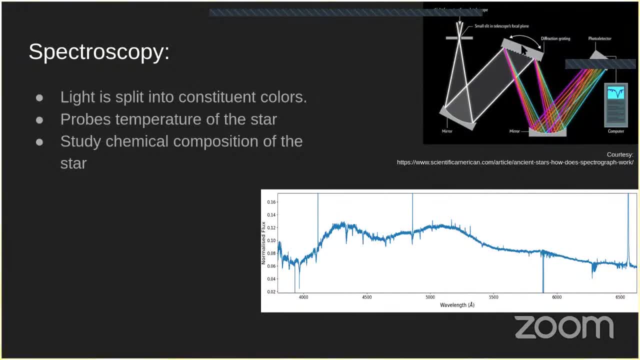 and then it's reflected onto something called as a diffraction grating. So diffraction grating is kind of an instrument that is used to split the light. So you can see that here in it is represented that the light, the white light, is split into. 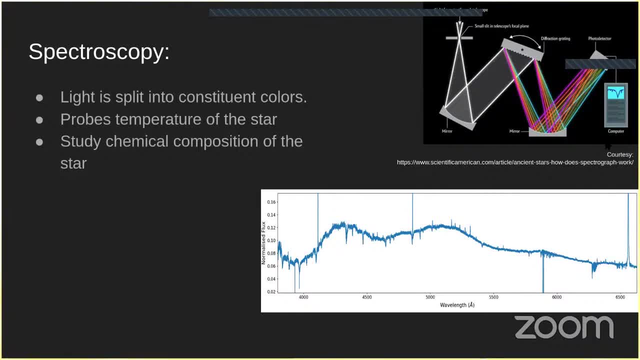 its constituent colors, And then so, and then the the detector, photo detector, just takes in those different colors and then it gives you. It gives you the spectrum- The one that I showed before was a 2D spectrum- and then you can convert that into 1D, which 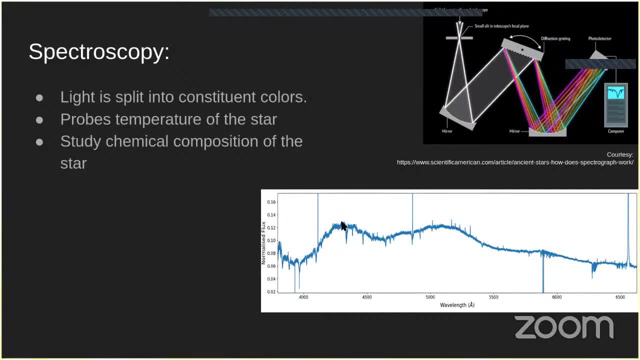 gives you a line plot and you can see there are dips. So these dips are the black lines that you see in the spectrum earlier. So you can see that there are a lot of dips. All of these are spectral lines which are formed due to absorption of light from different 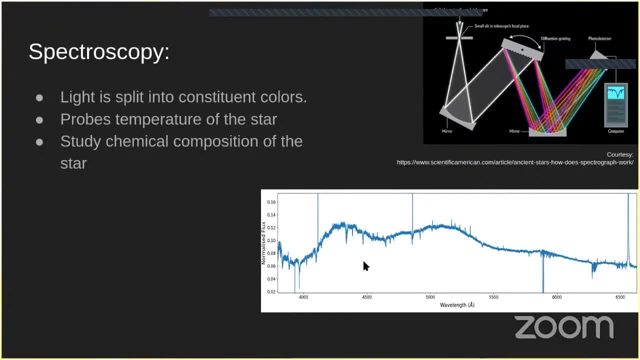 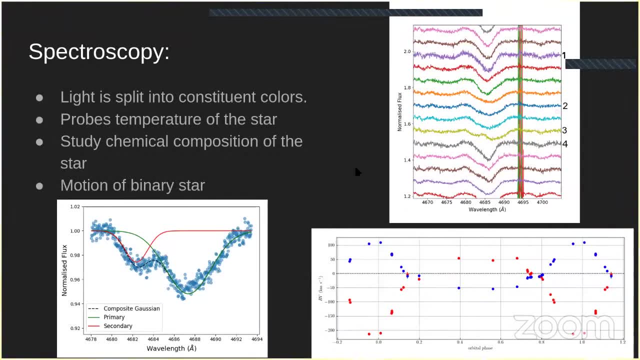 elements. You can study these in detail to know what kind of like, what kind of chemical, what kind of chemical compounds are in the star. The other use is to you can also study the motion of binary systems. So has explained binary system. 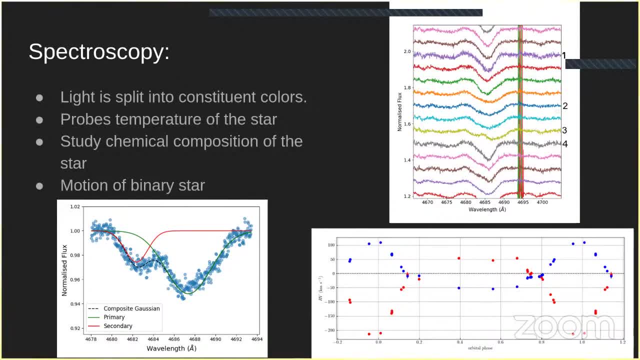 There are two stars moving around each other, So they keep going in us in a circle or an elliptical orbit. but this motion, because when there are going around one star, from your perspective, from art, one star is going away from you while the other side is coming towards you and this, this motion causes some. 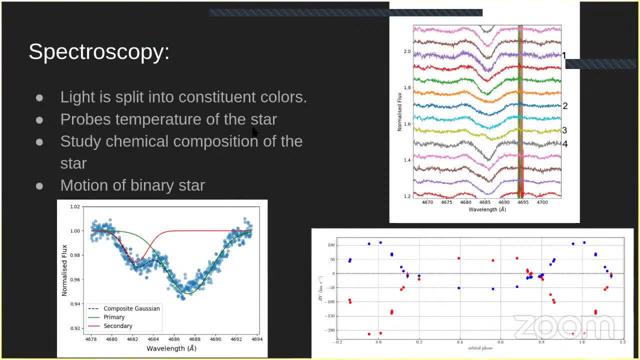 something called as redshift and blue shift. So certain wavelengths of the star going away from you is like redshifted, whereas the light of the star coming towards you is blue, shifted very slightly. So you can measure this. So here you can see an example of a star that's doing that. 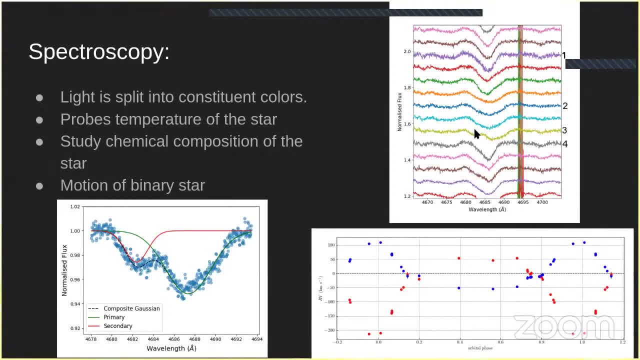 You can see that in some epochs there's just one dip, whereas in other epochs there are two dips. This is actually the same spectral line, but because these spectrums are observed in different point of time, the blue shift and redshift can be seen here. You can measure this using something. 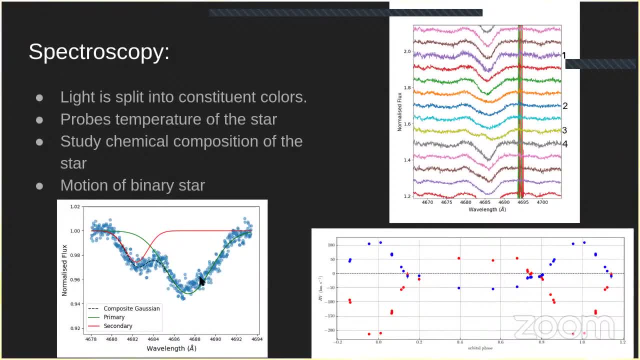 called as a Gaussian fitting technique. Here you can see that I have fitted two Gaussians into the same spectral line and I can measure the relative change in the wavelength and then calculate the velocity of the components. And here you can see that this is the wavelength of the spectrum. 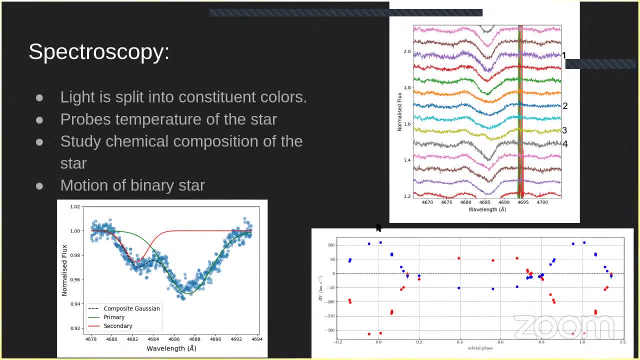 The radial velocity of the two components- The blue one is the primary and the red one is the secondary. So you can see that there is a motion like they reach a certain speed and then they come back. So you can use this to study a lot more about the system itself. Coming to gravitational 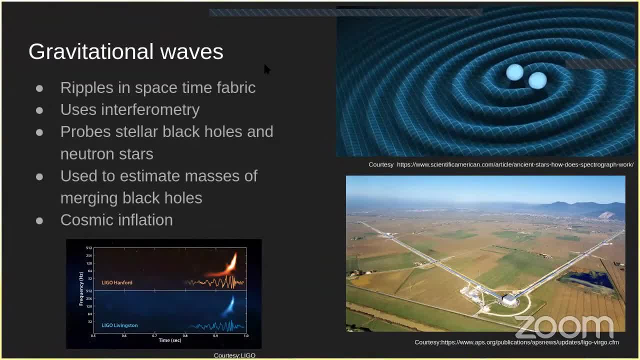 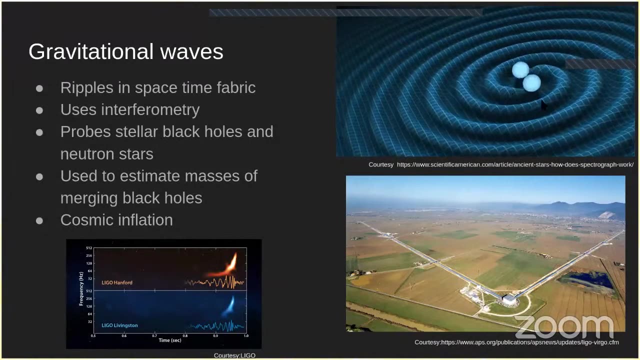 waves. as mentioned, gravitational waves are nothing but ripples in the space-time curvature. Here is an a representation of what. So here they are showing two neutron stars going around, But this also holds true for black holes. So when they go around, they form these ripples. 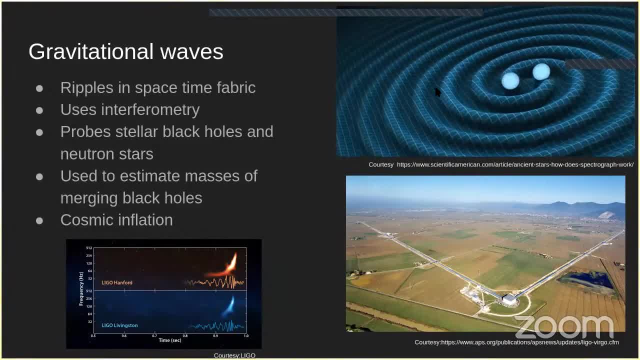 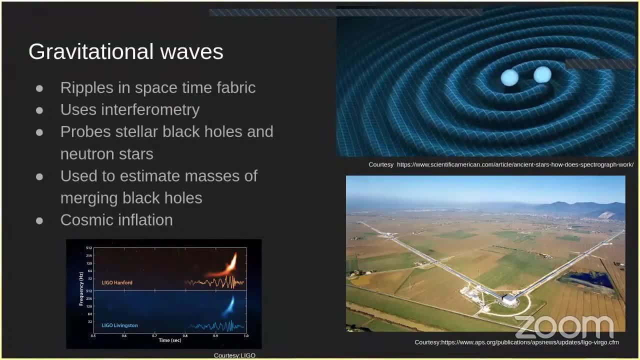 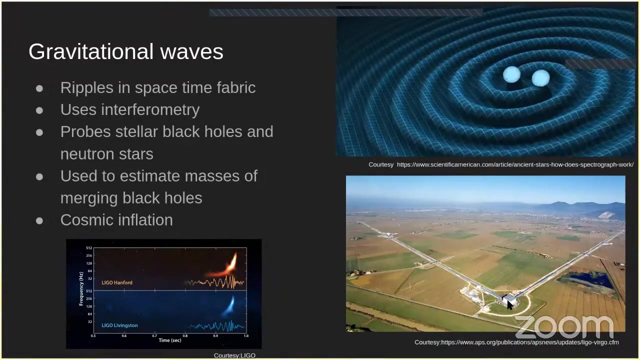 and these ripples travel across the universe and when they come to earth, you can detect it. But because these ripples are very, very, very small, the magnitude that you are dealing with is extremely small, So you need a very, very accurate detection technique. So there are three observatories currently working called LIGO and Virgo, So there 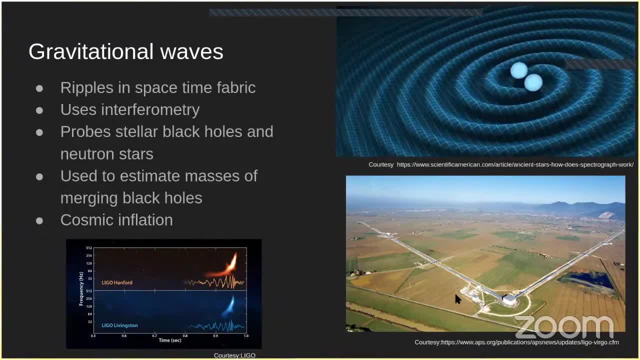 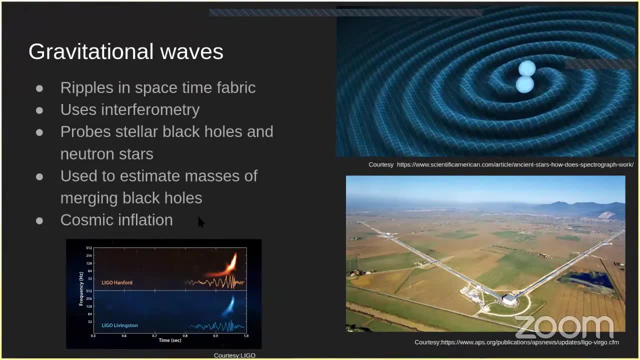 are two LIGO at Hanford and Livingston and one more in Italy. It's called Virgo. LIGO stands for Light Interferometer Gravitational Wave Observatory. So this is the observatory. You can see that there are two arms which are perpendicular to each other. Each of these arms is four. 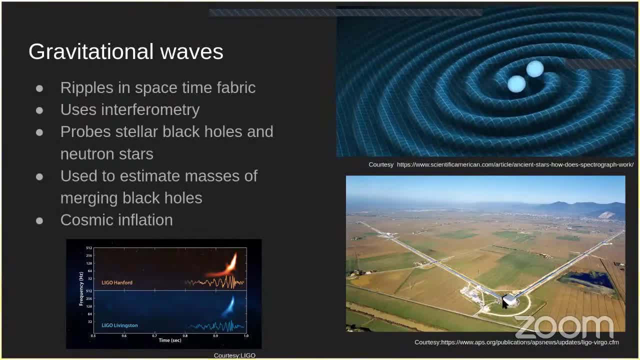 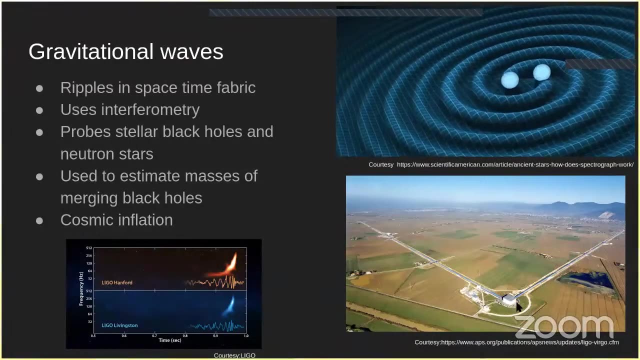 kilometers long. So what it does is, again, it uses interferometer, interferometer technique. So there is light that goes in one arm and then it's reflected back into this uh station And same happens in the other arm also. But when they come down, They are uh, they. 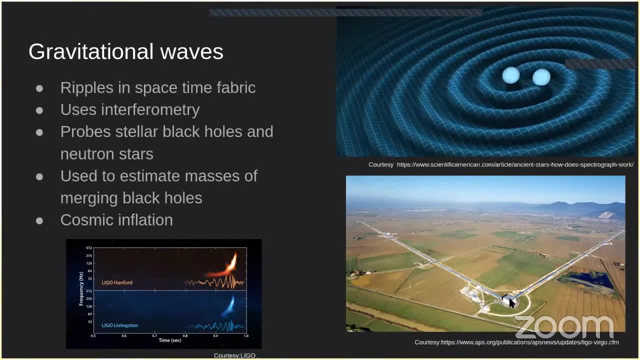 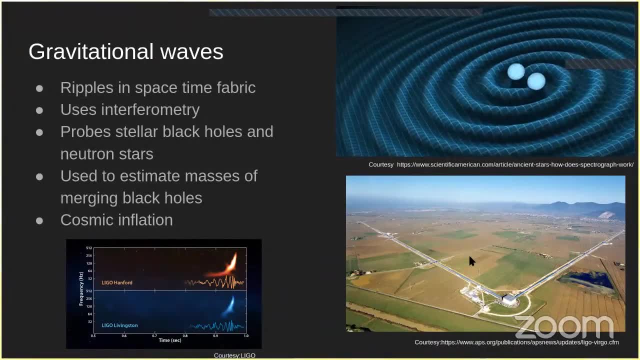 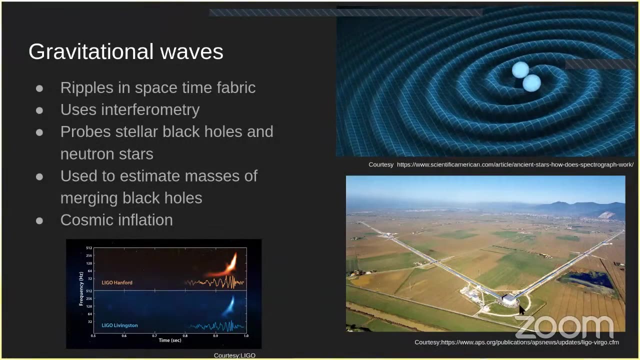 interfere with each other, either constructively or destructively. but when these ripples come to earth, The earth, all the, the, the, the, the, the. the circumference of the wings of the shape of the earth also changes, because the space-time curvature itself is changing And this change in the 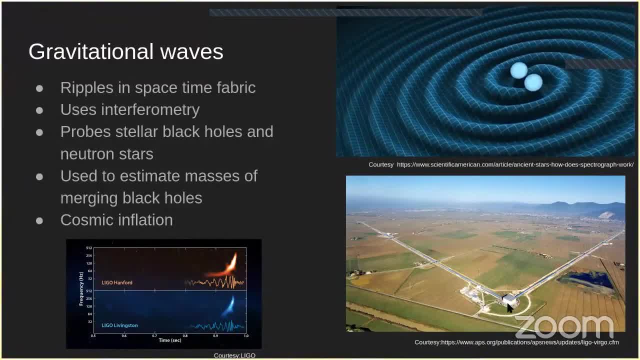 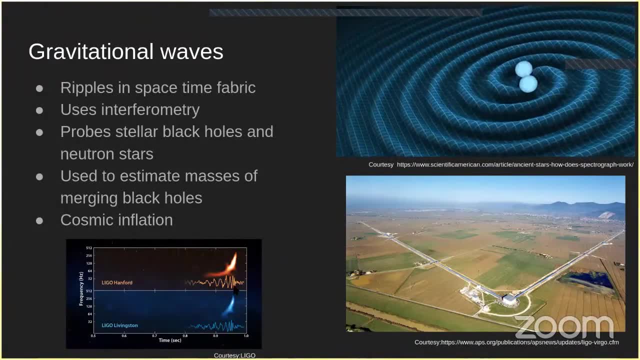 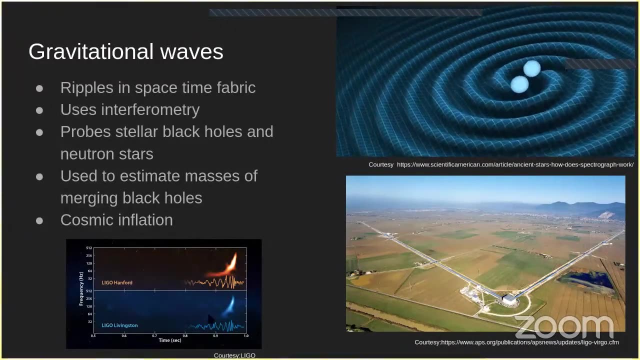 curvature itself will change the interference that's happening. So you will kind of get a signal where you can see that there is small and then there's a large changes in this interference of the light in the two arms. So you can do this and then see if you have actually 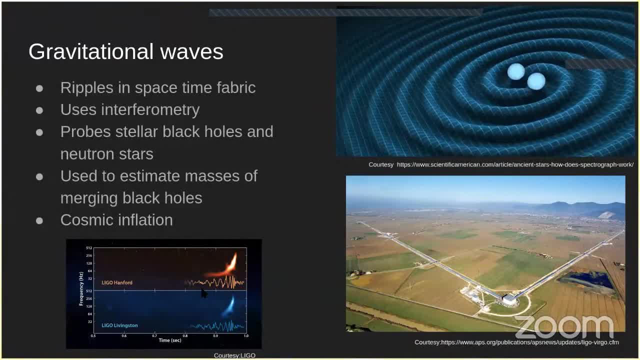 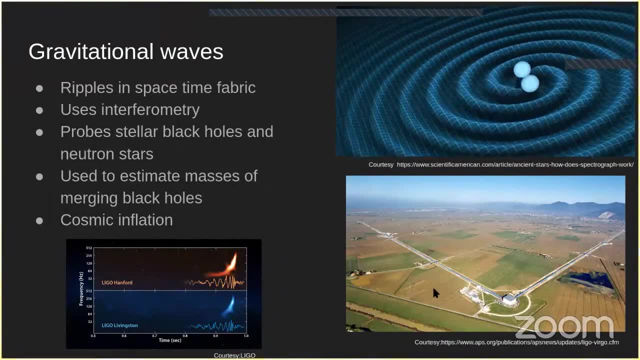 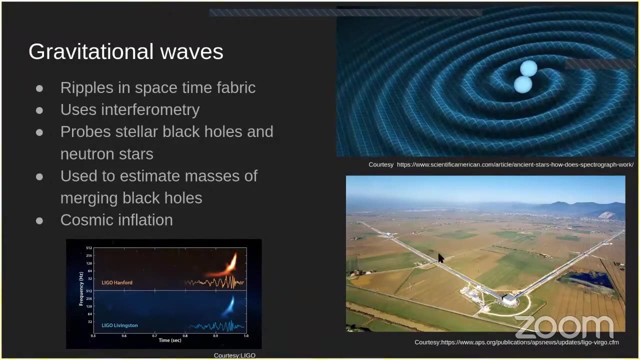 detected a wave. Again, this is a very simplified version. The actual thing that takes place is much, much more complicated, because the changes are so extremely small that they have to take everything into consideration. Even like a man walking near these tubes can affect the results. 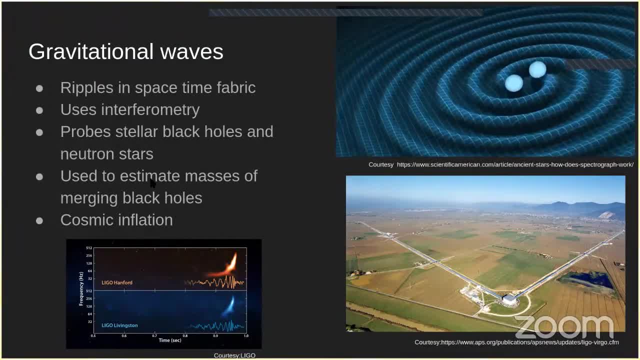 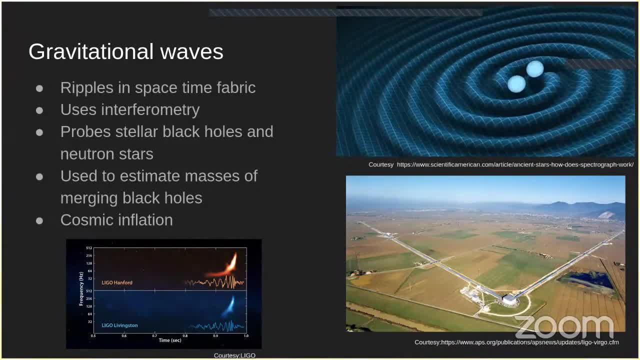 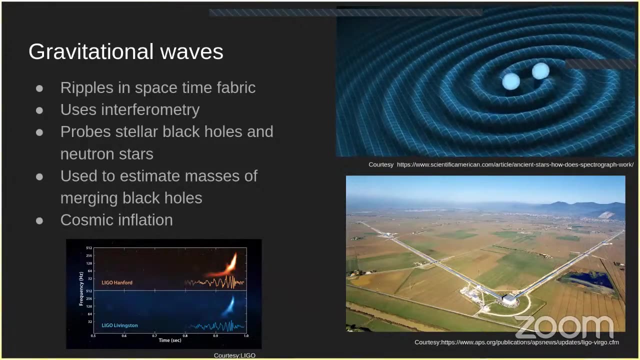 So you can see that the waves are very small. So you can see that the waves are very small. So in the early universe there is a concept called cosmic integration, where we think that universe expanded very rapidly in a very short period of time. So if that took place, 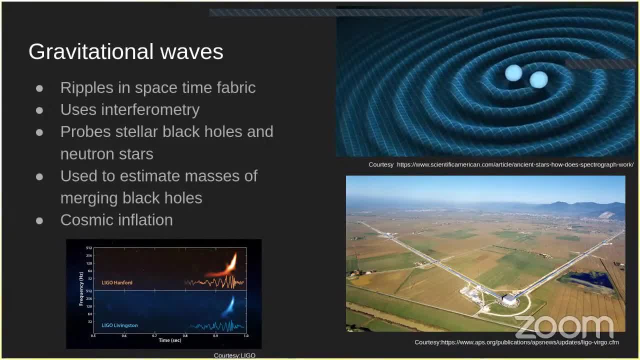 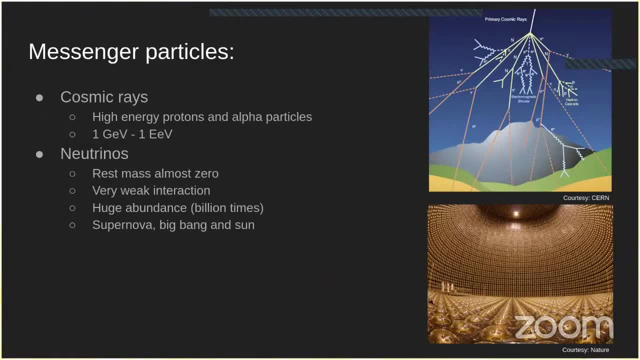 then there should be gravitational waves originating from them and you should be able to detect it now. but yeah, that is what astronomers are working towards currently. Coming to messenger particles, this is the last technique that we are going to discuss. Messenger particles are nothing but. 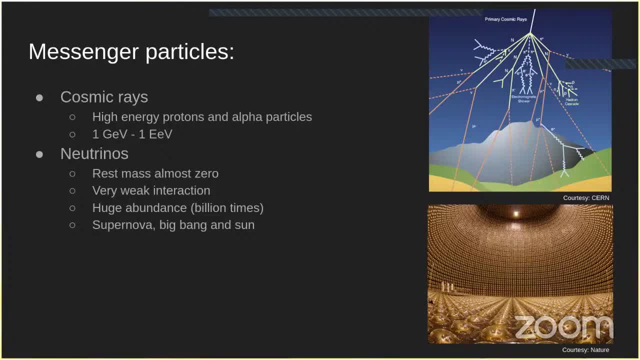 so, as the name suggests, these are particles which bring information to us. There are two important messenger particles. one is the cosmic rays and another is the neutrinos. Cosmic rays are nothing but high energy protons or alpha particles. Alpha particles is nothing but the. 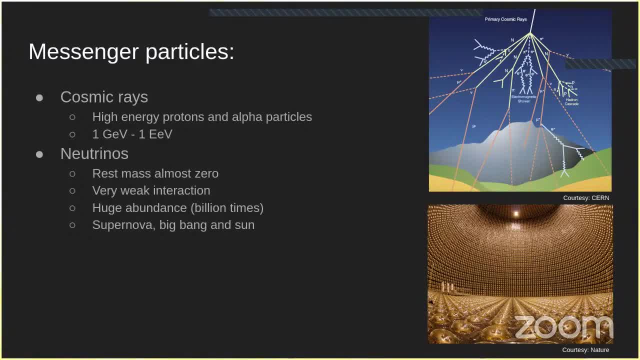 nucleus of a helium atom. So these are very high energies. The energies can go from one giga electron volt to one exa electron volt, which is tremendously high. So when they come and then they hit earth again, just like gamma rays, because of their high energy they form a cascade of 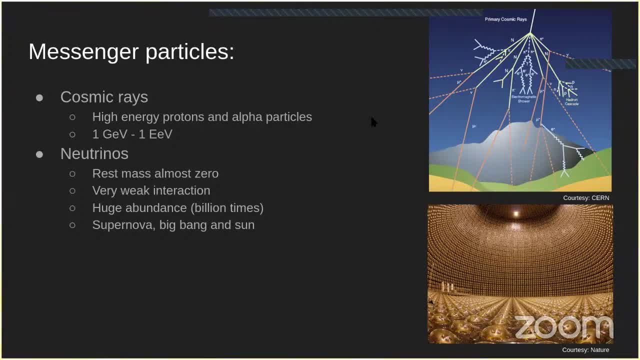 showers, which is in this case it's called air shower, where they hit many different particles and then they form a shower kind of thing. You can detect this shower, just like you did for gamma rays, and you can estimate where it came from and all these. 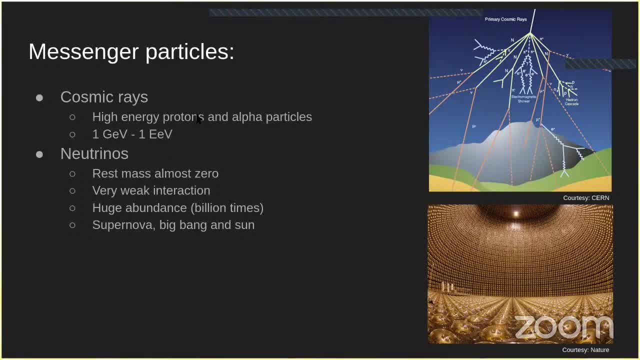 Some sources of cosmic rays are the sun itself, supernova remnants and certain energetic events like AGMs. The second one is neutrinos. Neutrinos are fundamental particles which so they are so light that the rest mass is almost considered to be zero, and because of this they also have a very weak interaction with matter. 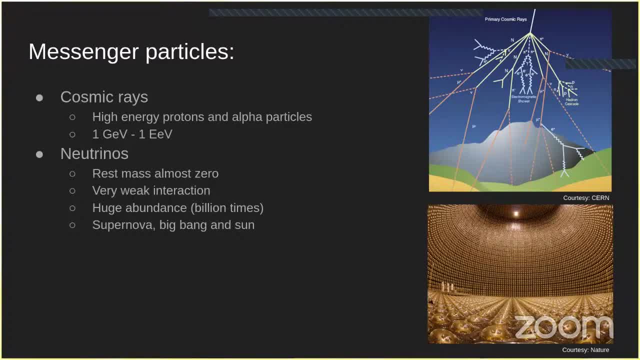 So they rarely interact with matter, which makes it that much more difficult to actually observe this. So how do we observe neutrinos? You can see an example of a Japanese observatory called Super Kamiokande- I'm sorry if I didn't pronounce it right, So this is a kind of a tub. 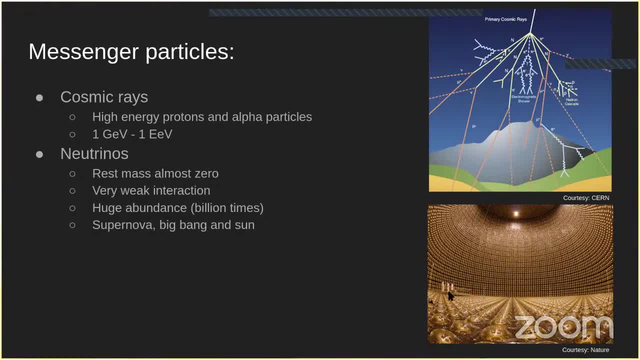 This is a upset tube kind of a region where it is filled, so you can see the extreme size of this tube. right, these are humans standing here and then this is like the size. So they fill this tube with like ultra pure water and then these golden things around are like photo detectors. so 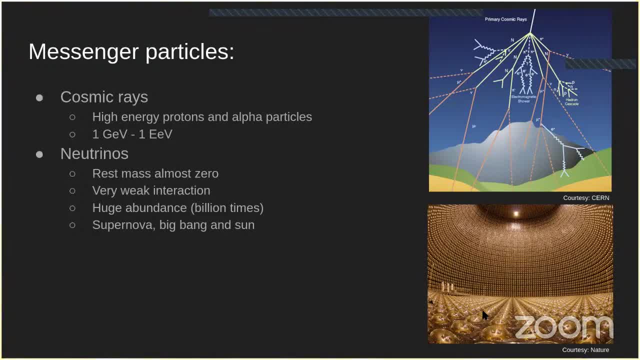 they detect even the slightest change. So when a neutrino comes, because of its speed it kind of of it gives out a certain light and then these photo detectors can detect that light and they can estimate how much, how many observations are made, even though such a big facilities available. 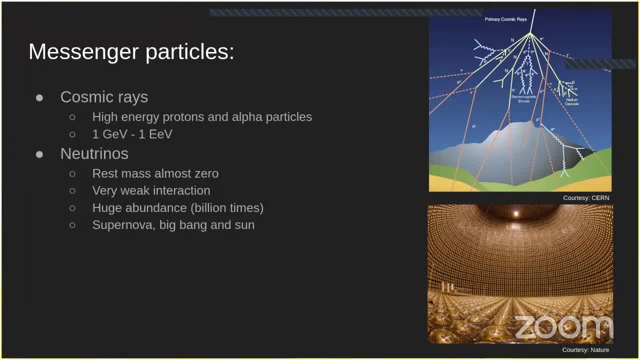 the number of neutrons detected are very, very small because they interact, so so less, yeah, so again, these are formed again in the supernova and sun, and these kind of give you an estimation of of what's happening in the early universe as well, because even big bang. 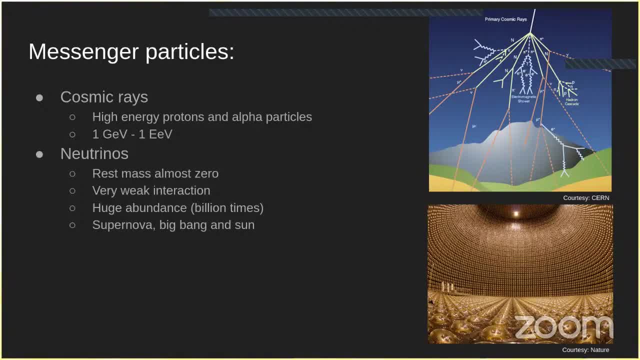 would have produced some neutrons. so that was a brief discussion, brief session about different techniques that is used. someone can either use one technique to do some research, but usually, in majority of cases, astronomers use multiple of these techniques in together to kind of have a really good results at the end, which is which is which is useful. 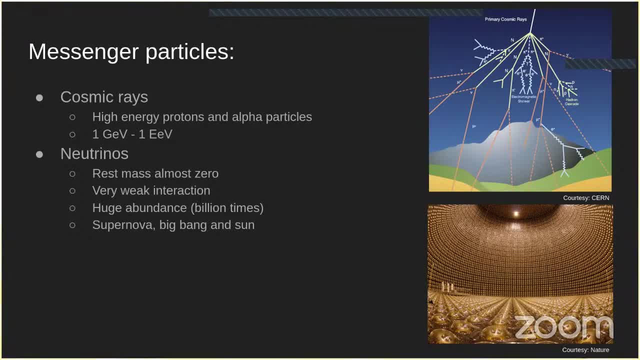 i hope this kind of gives you an overview of what observation astronomy is like and hopefully it kind of encourages you to pursue this, this stream. yeah, thank you, that was my presentation. uh, if anyone has questions or anything, if you want to ask, then you can just ask right now. 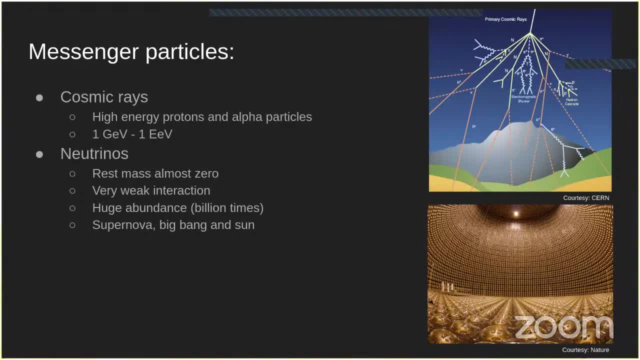 i don't think there's any questions. hello, is someone there or am i just talking to myself? yeah, no questions such as: but thank you, hey, nagraj, hello, yeah, so, uh, thank you very much for this uh very wonderful session. it was very nice and, and uh, does anyone have any questions? guys, it's very nice to see you. thank you very much for this uh very wonderful session. it was very nice and and uh, does anyone have any questions? guys? it's very nice and and uh, does anyone have any questions? guys? thank you very much for this uh very nice and and uh, does anyone have any questions?